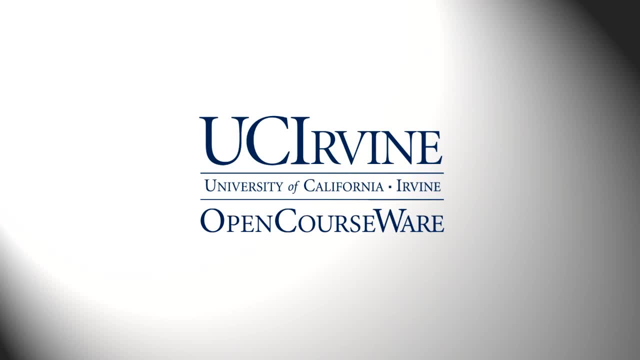 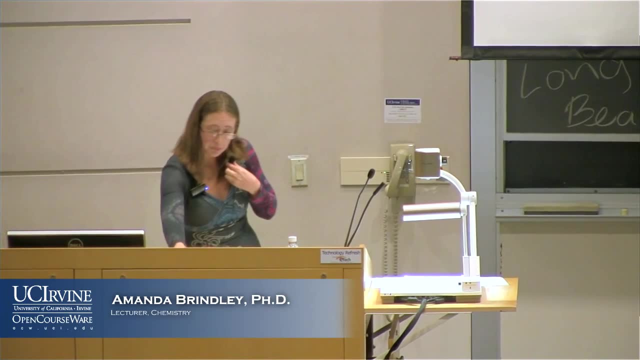 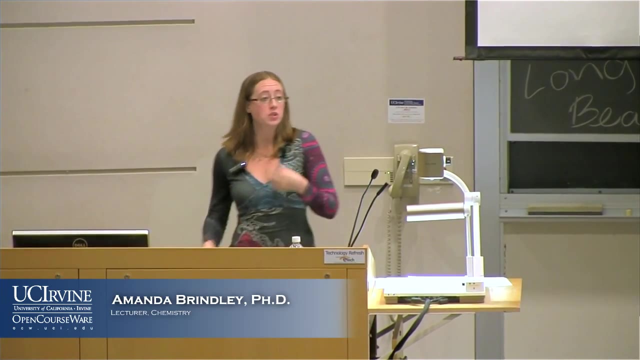 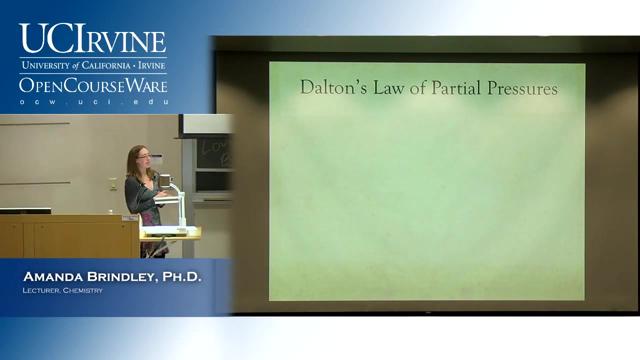 Okay, so today we're going to pretty much. let's see. alright, I think that's better. Okay, so today, if you guys can be quiet, we will. Okay, we're going to kind of start back and talk a little bit more about Dalton's partial pressures. I think really we'll spend. 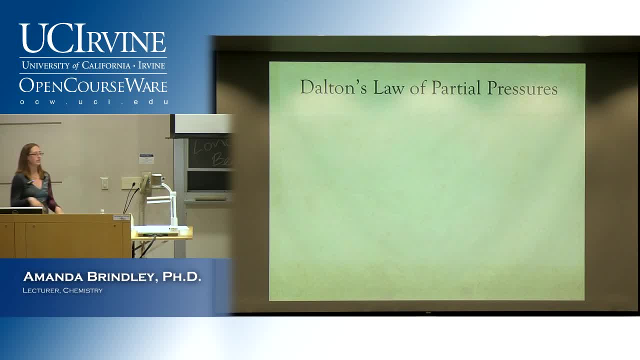 most of today on doing the various versions of this and the various examples, because it is a little bit long. We may make it into a fusion, So I'm hoping to finish up the gas laws on next Monday and then be able to spend Wednesday and Friday on review for you guys. I think two review lectures would be best, but it really 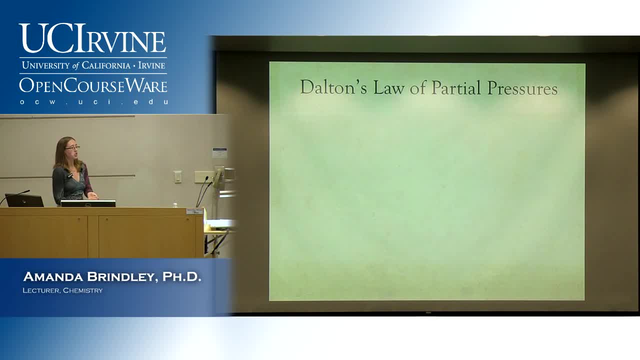 just depends on if we can make it through or not, And I'm not 100 percent sure if we will or not. So, without further ado, we'll get going. So review a little bit from the last five minutes last time. So remember that partial pressure, the way that this works, the way that this 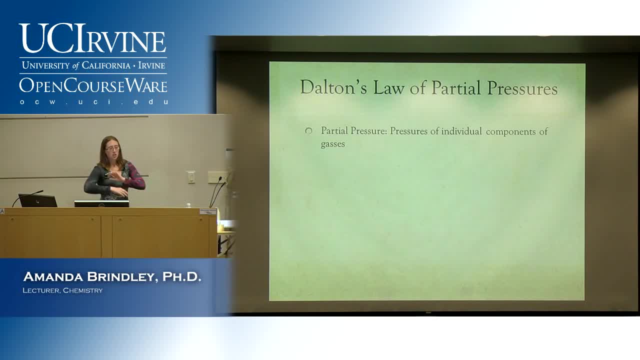 works is that you can take the pressures of each individual gas. So let's say you have a mixture of three or four gases. You can take the pressure of each one of them and then add them together and that will give you your total pressure. 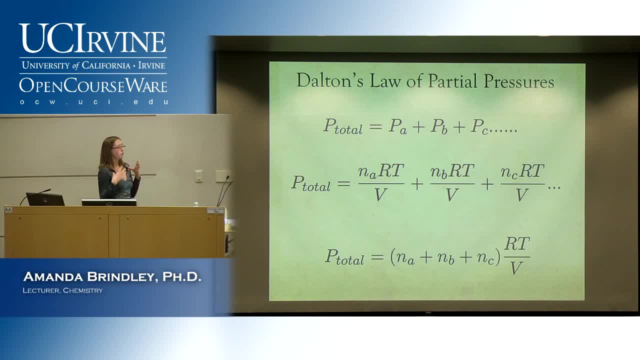 So when we did this sort of with an equation form, this is written out. So this is written out in just: pressure of each gas equals pressure of the total. So using the fact that we know that pressure is equal to NRT over V right Ideal gas law. 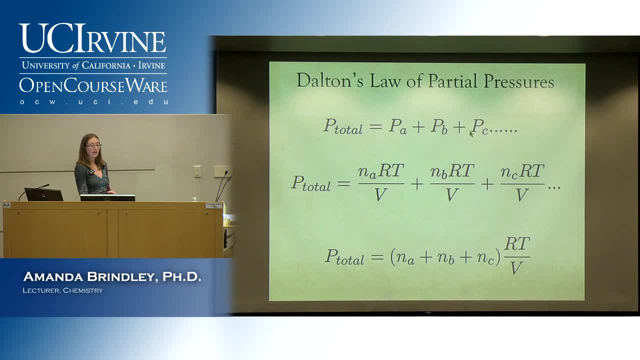 We can take and we can solve the pressure for each individual gas and then we can add them all up together And we know that if we have a container with a mixture of gases in it, that the temperature and the volume are going to be the same. So we can go ahead. 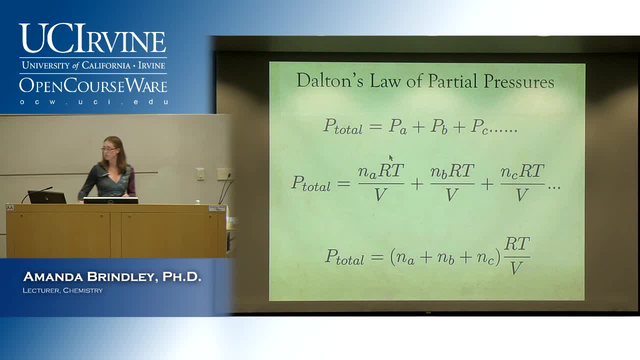 and we can pull that out, We can factor the moles out and then we can get this. So what this really says is that you add up all of the moles and you can add that up and then you get your total pressure. So your moles of all your gas, you can fill it right into your ideal gas law as well, and 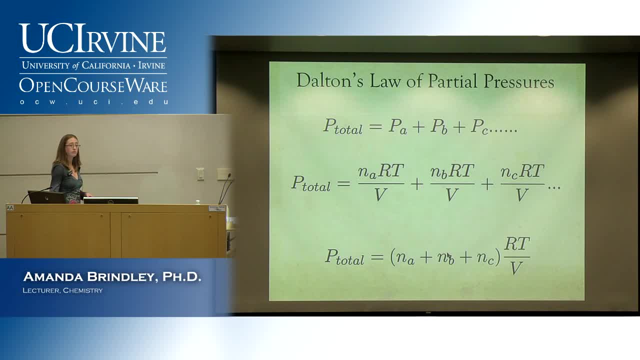 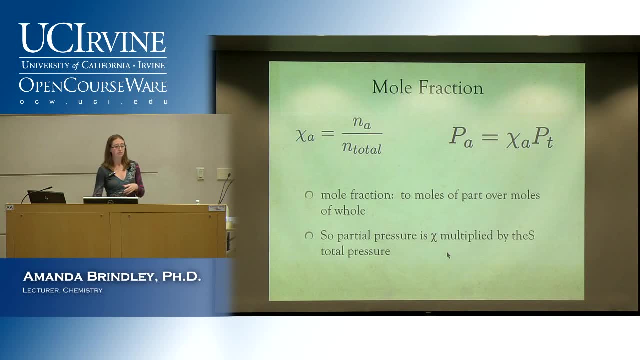 solve for your total pressure that way. So two different ways of doing it. Now, there's a very important concept here that we need to talk about, And that's called the mole fraction. So this X, this is actually the Greek letter chi, So that's how you say that. 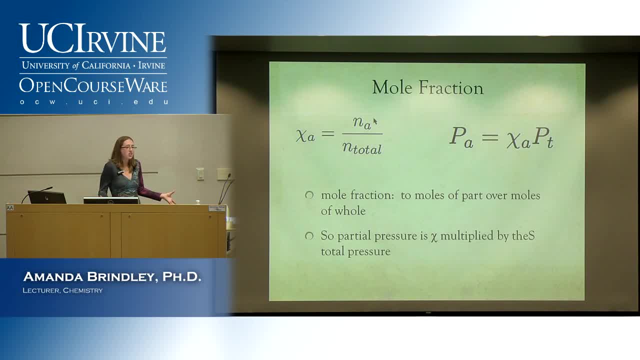 And this says that if you have the all, this really is a fraction just like any other fraction, right Yeah, It's a mole over top of the total. So if you want to know the mole fraction of A, you put take the moles of A and you put it over top of the moles total. It's no different. 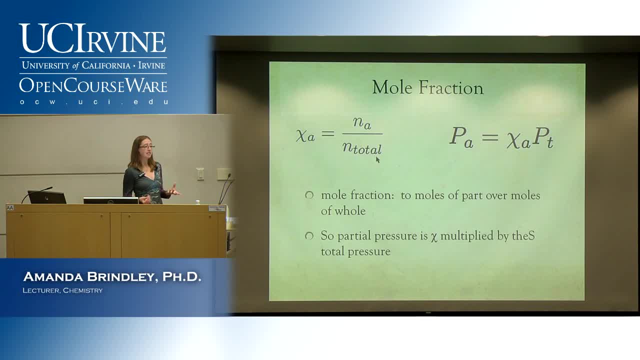 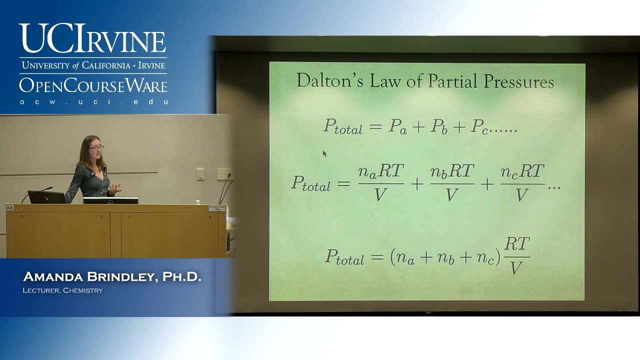 really than saying the percent of A like the mole percent of A, except that you don't have the times 100 percent there, It's just the decimal point or the fraction. So that's what mole fraction is. Now what this says is it kind of takes this concept combines. 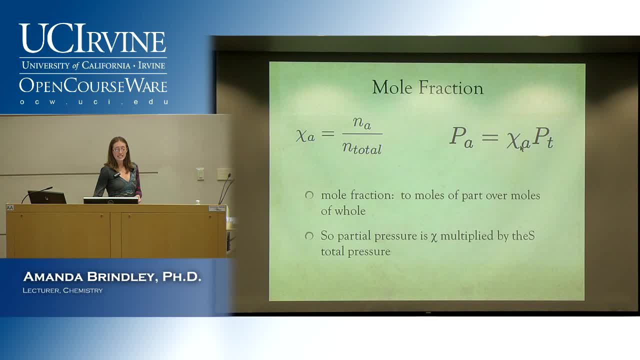 it with this one, Okay, OK, and says, well, we can take that chi, we can take that mole fraction right our part over our whole, and we can just times that by the total pressure. This isn't any different than the sort of how you work with percents your entire life. 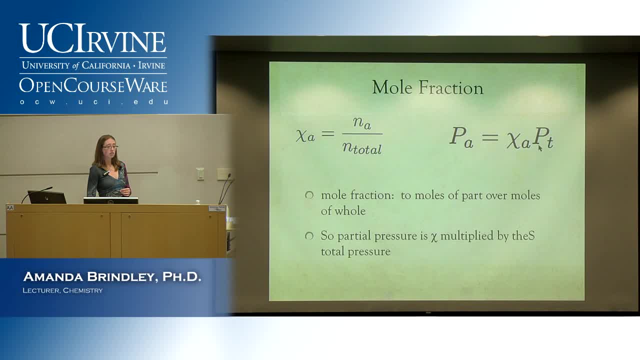 right. If you want to know what percent something is of a total, you take the fraction and you multiply it by the total. OK, So this is your total pressure. So if I tell you that something has a total pressure of 5 atmospheres but the mole fraction 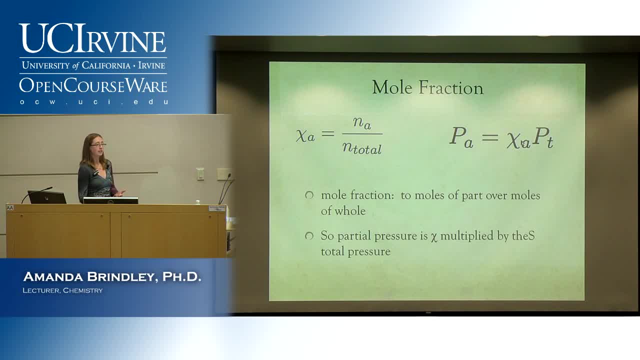 of it is only 0.2,. take 0.2 and times it by 5,. OK, So don't let this seem like a new equation to you. This is just using percents, like you've always used them. except what's the first thing you 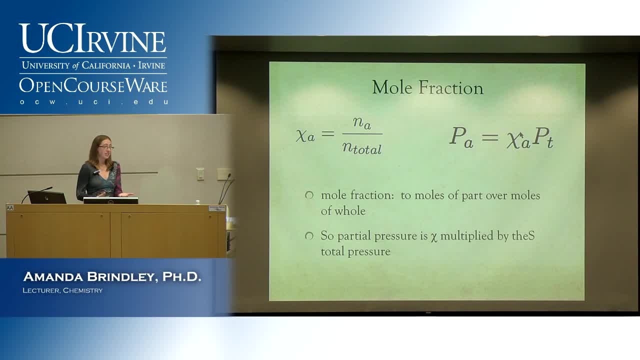 do. if I say you have 75% of something, You turn it into a decimal right. Well, that's all this is. It's just the decimal of the part over top the whole, So that's all mole fractions. It's like a percent, except not with the percent. 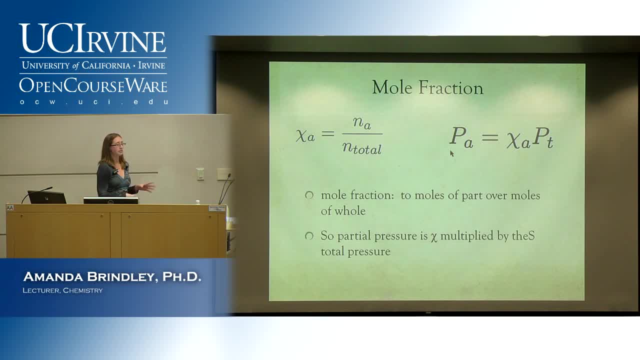 I'm not sure why they go through the you know special aspect of naming it different and calling it chi and all of that. but you know that's fine, So don't let this be new to you. Just kind of a different way of naming it. 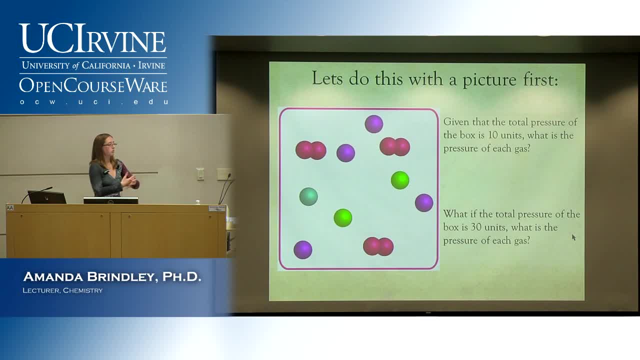 OK, So before we do partial pressures with actual numbers, let's just go through and do it with a quick picture. So if I have this and I have this mixture of molecules, So I have some purples and some greens of aqua or cyan and some pinks. 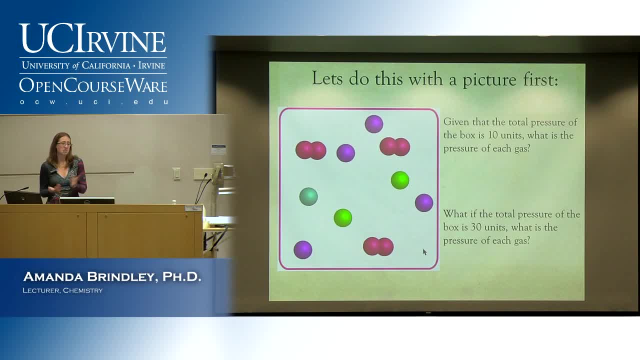 If I tell you that this has a pressure of 10, it doesn't matter what unit, I say 10, and we want to know the partial pressure of each gas. what do we do? We have to find the mole fraction, right? 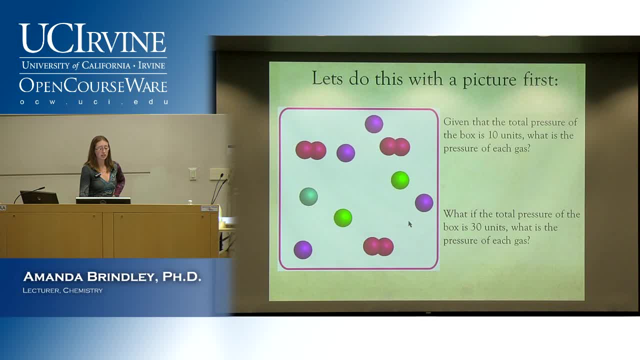 So let's start with the purple ones. So first of all let's figure out how many. what's our total number of molecules, or total mole of molecules? So our total number of molecules, we just count. OK, One, two, three, four, five, six, seven, eight, nine, ten, right? 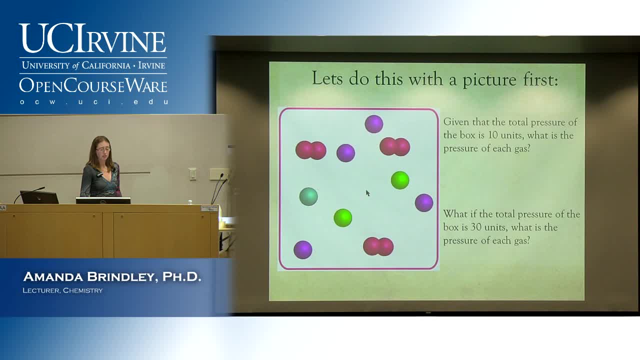 Now, if we want to know our mole fraction of the purple ones, what do we do? Well, how many purple ones do we have? And I apologize for the color blind people. Statistics say there's at least a few of you, and I do apologize. 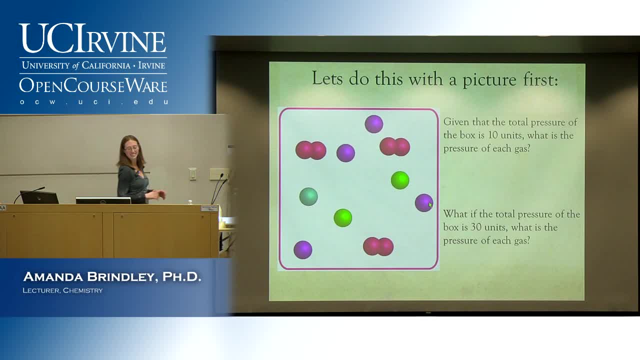 One, two, three, four. I won't do that on an exam, obviously. So there's four out of ten, right? So your mole fraction is four out of ten. So, OK, What would be our mole fraction of the pink ones? 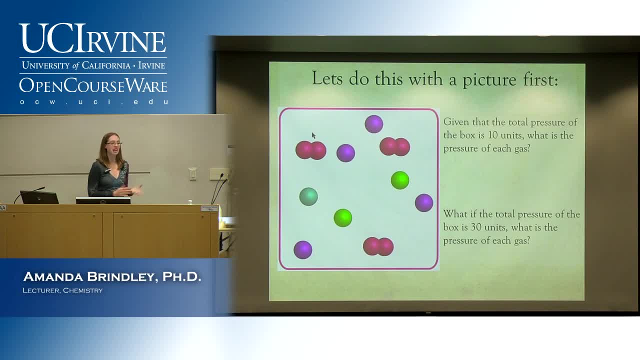 Would it be six out of ten or three out of ten? Good Three. It doesn't matter that it's a diatomic right. We're treating all of these molecules and all of these atoms and all of these gases as just like they're just spherical balls that are all the exact same. 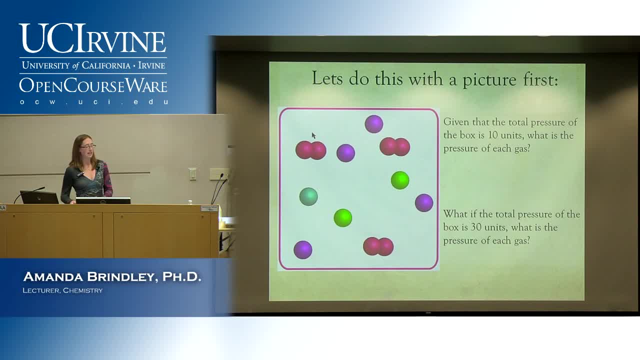 They have no volume, They have no interaction, They have nothing. They're just ideal gases. So it doesn't matter if I drew these as diatomics and these as single, So it would be three out of ten right Now. so what does that mean? 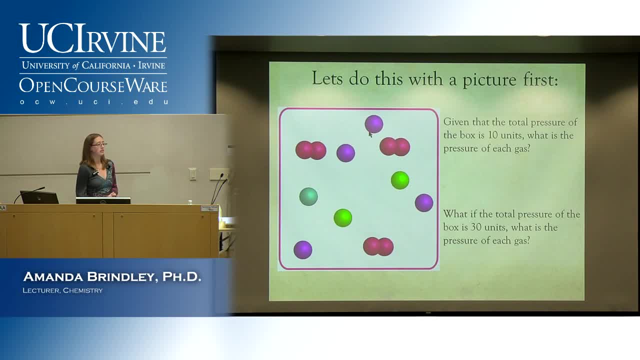 The pressure of the purple ones would be four out of ten. So just four, right So? and you can go through. You can do that with each one. So the blue would just be one out of ten. That would be your fraction. 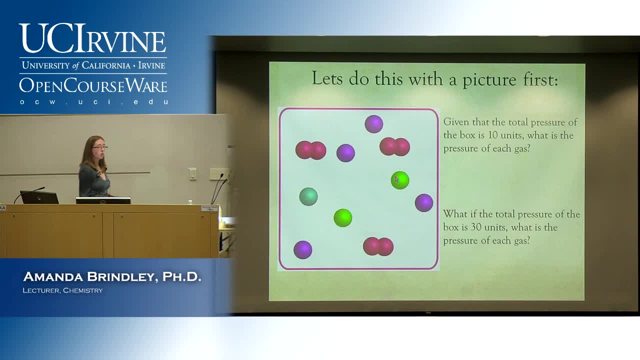 It would be 0.1.. The greens would be two out of ten, 0.2.. So all mole fraction is is a count right. It's how many moles of something you have. In this case, how many atoms works the same either way over half of the total. 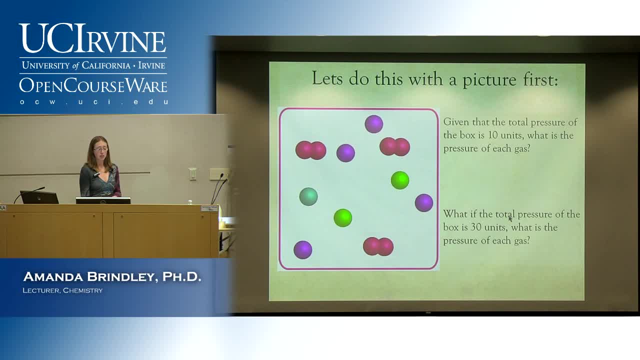 So now if we were to go through and say, Well, what if the total pressure of the box is 30 units, Then what would it be? So it changes things a little bit right, But not too much. So I'm going to have to flip over to the document screen for this, so we can write. 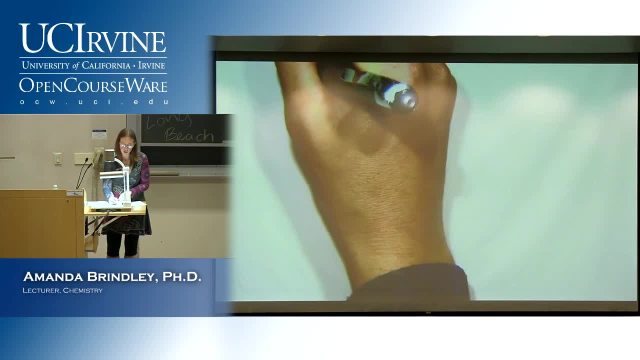 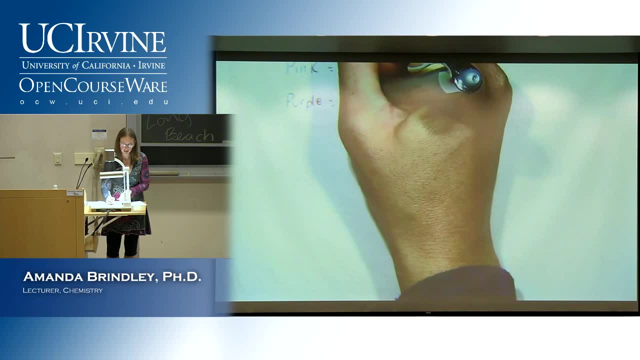 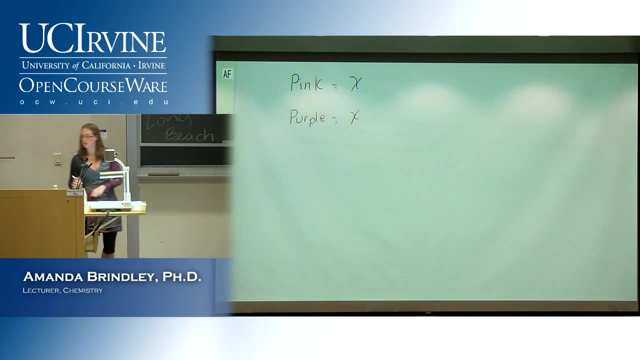 So let's just do this for a couple of them. So we talked about the pink and the purple ones and we talked about chi, So let's write it down. I would suggest us doing this right on the slide. that's why I didn't put it on the worksheet. 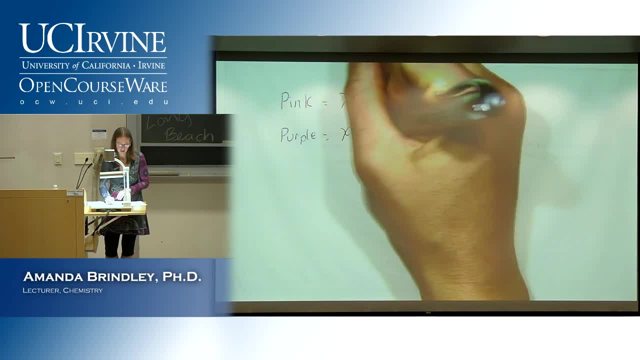 So we have our pink, we have our purple. What is our chi for each one? So you're looking at your picture, and for the pink, we had said, well, there's 3 out of 10. and for the purple, we had said 4 out of 10.. 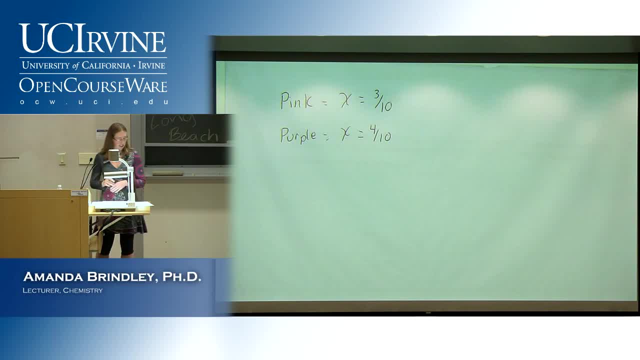 All right, so let's just do it for those two. I'll say that you can do the green and the blue at home. So now I said: well, what if the total pressure is 30? 30, whatever? Because we're talking about molecules and not moles, it's kind of odd to use normal units. 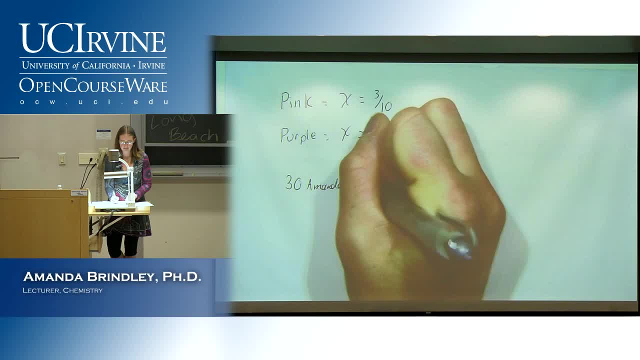 So we're going to call them 30 Amanda units. What is going to be our pressure, our partial pressures? How do we figure this out? Well, it's just a percent, right? You're just treating this like a percent. So if we want to know our partial pressure of each one, 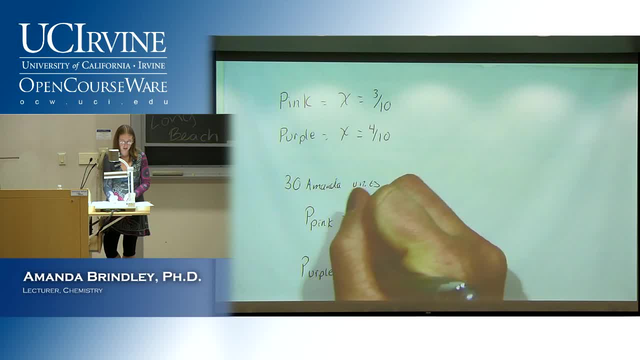 Okay, We take our mole fraction, we multiply it by the total to get our answer. If we took our purple, we would do 4 out of 10 and times it by 30 to get our answer. It doesn't matter that I, you know, I drew one as sort of kind of your ideal gases, right? Helium, neon, whatever, Because it's just mono-atomic And your other is diatomic. You just take the mole fraction, multiply it by the total and you're done. Okay, So part Dallin's Law is really nice. 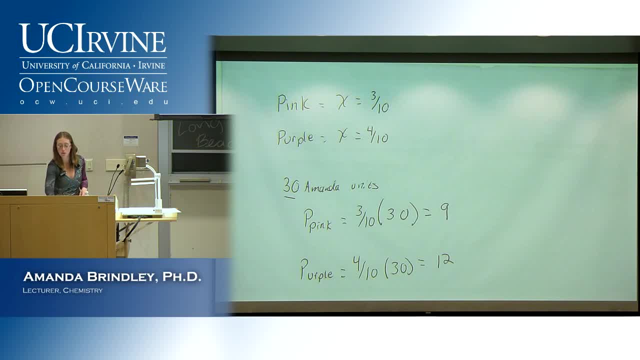 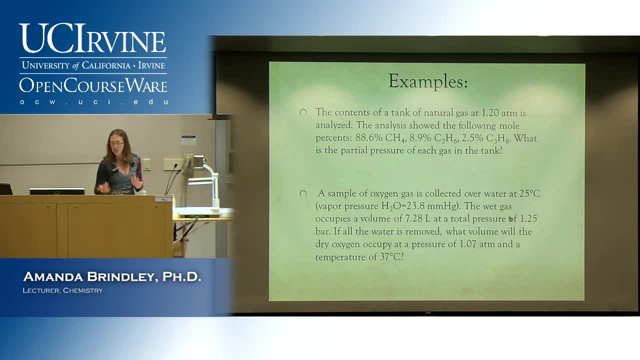 It makes life kind of easy for us compared to if that, if all of this wasn't true, Okay, I guess I didn't need to switch over. Now we're going to do some examples, So the best way to do these is really just tons and tons of examples. 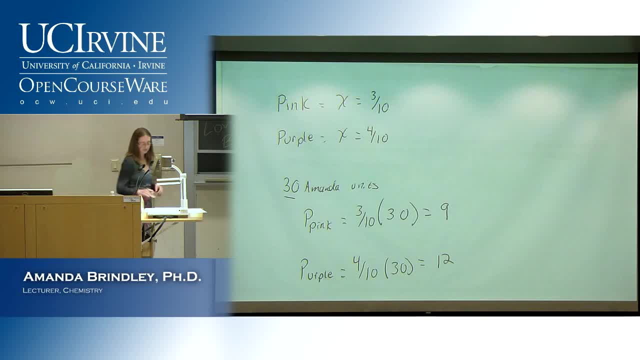 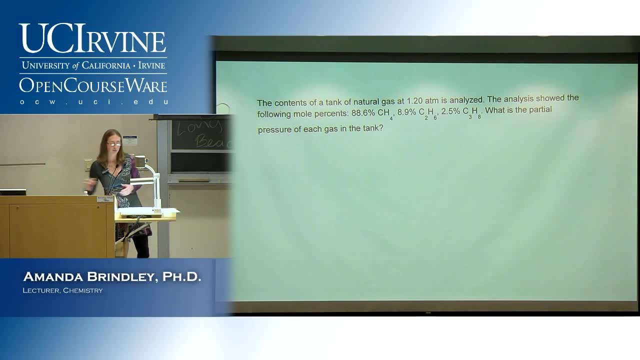 It's kind of the common theme for the majority of this lecture. Okay, Okay, Okay. So we have this. You have the contents of a natural gas tank, right, Because natural gas can be a whole variety of gases, It's not just one, one thing. 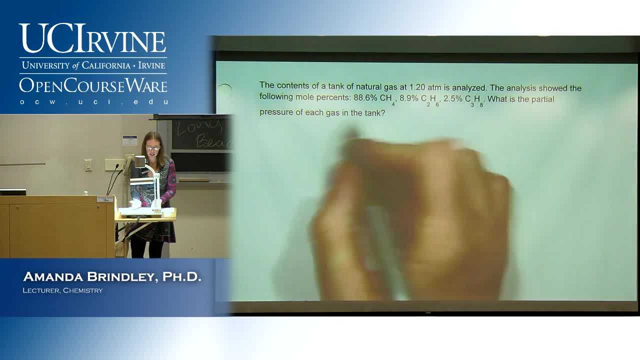 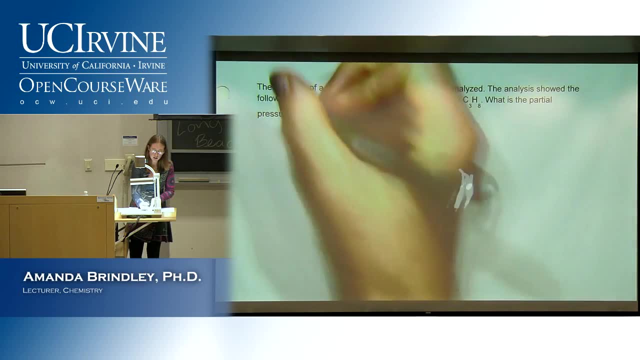 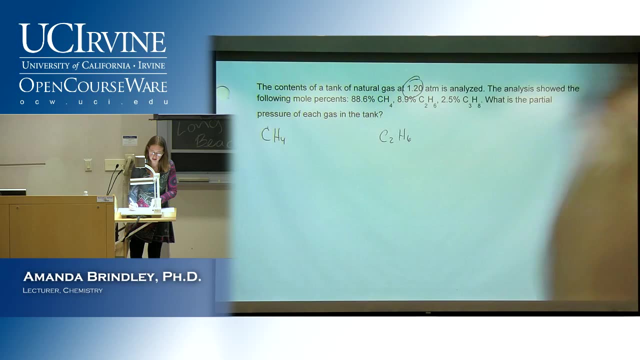 And I give you the percentages of each one And I say: well, what's the partial pressure of each one, Given that the total pressure is 1.2.. So let's break each one up- C2H4,, C2H6, and C3H8- and we need to figure out the partial pressures of each one. 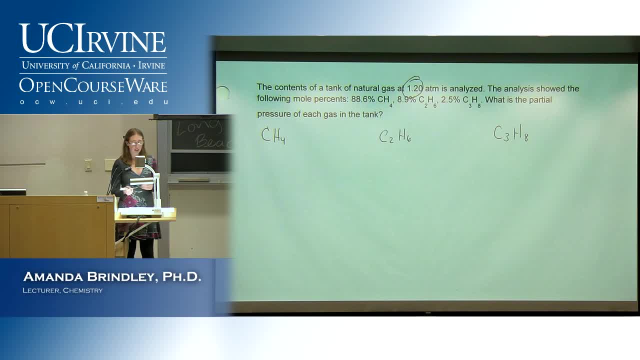 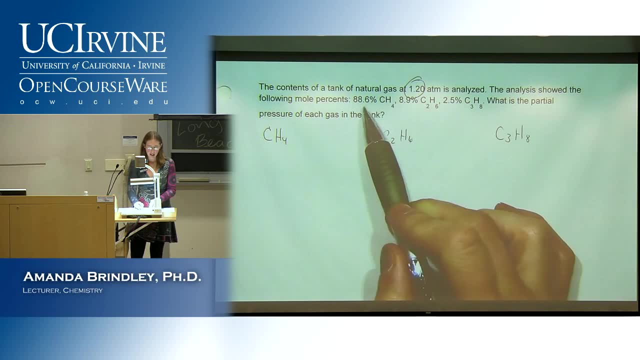 So how are we going to do this? Well, this time I didn't give you a mole fraction, right? What did I give you? Percent, Percent. So are we going to take 88.6 and multiply by 1.2?? 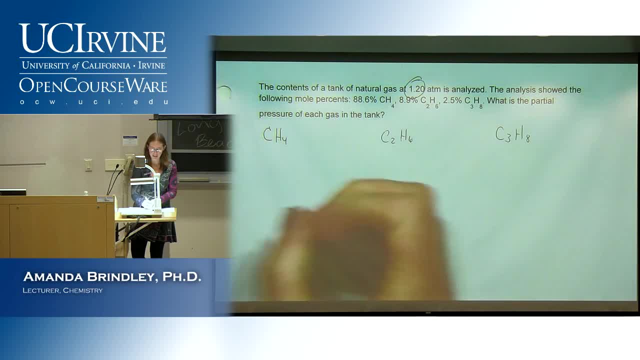 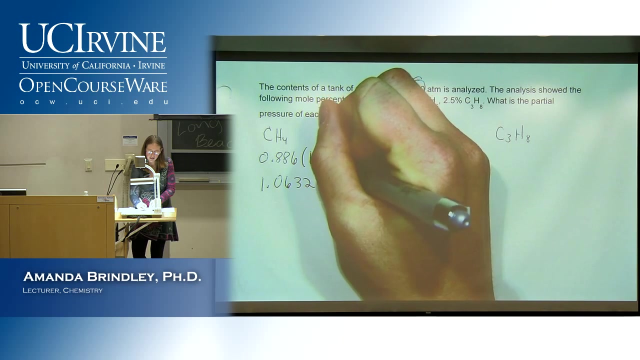 No, What do we have to do first? So we'll convert that and multiply by 1.2 to get our answer. So we get this and just for sig fig purposes we need to add that zero in there. So we need to round this to the three sig figs. 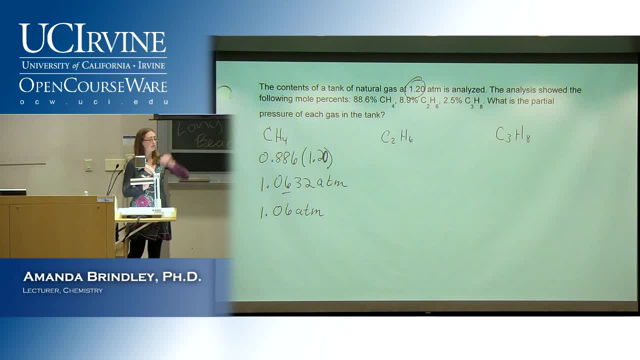 And we have that. OK, Yeah, Would you ever ask us like, oh, what's the partial pressure of carbon in CH4?? You mean, OK, no, so I couldn't do that because the carbon itself wouldn't be a gas. 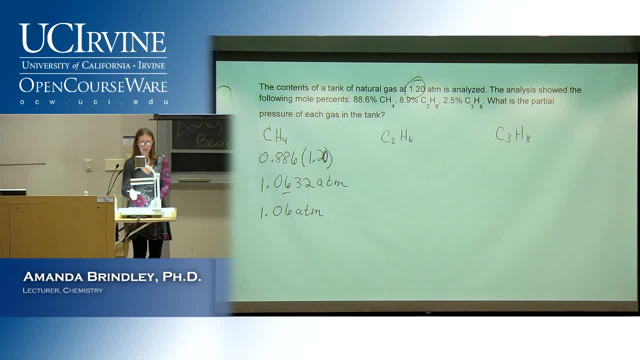 I could ask you for the moles of carbon, which, if I did that, you could take this, and how would you find moles of CH4?? You'd have to fill in the ideal gas off, so I'd have to give you some more information. 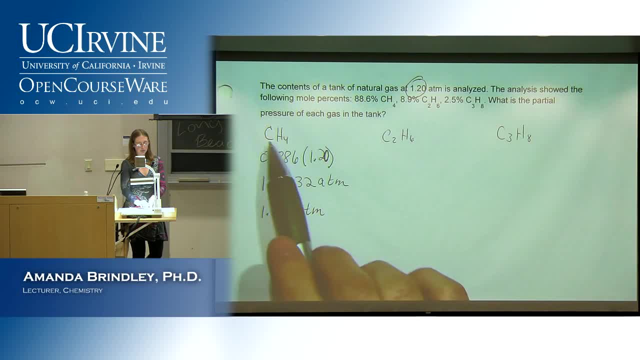 right, The temperature, things like that, And then you would know that however many moles of methane there is, how many moles of carbon would there be One? So I can go to moles of the individual elements, but I can't go to a partial pressure of it. 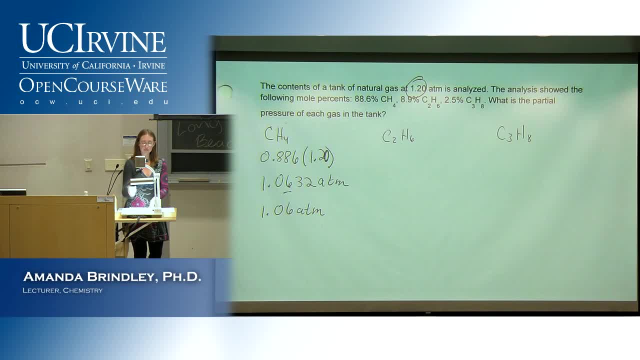 It doesn't make a lot of sense to talk about. OK, this one. So we convert that to a decimal. Careful with your single percent. Sometimes people miss the second, moving over part of it. So we multiply by the 1.20 atm to get our answer. 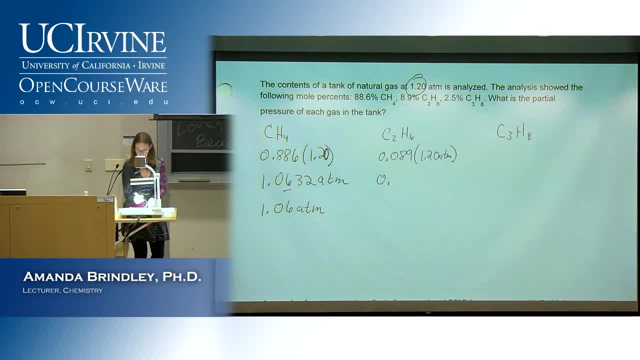 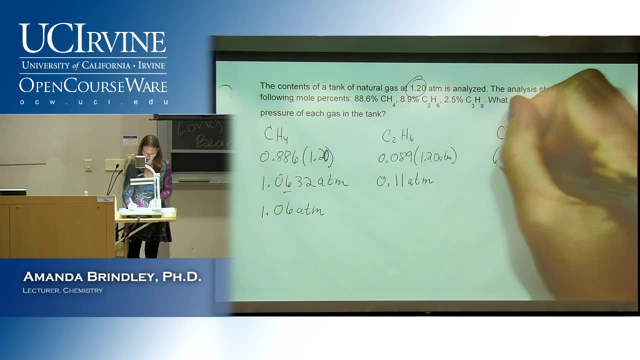 And we round to three sig figs, or, excuse me, two sig figs this time And our last one. So once again, OK, OK, OK. So we convert to a fraction. We multiply by 1.2 atm. 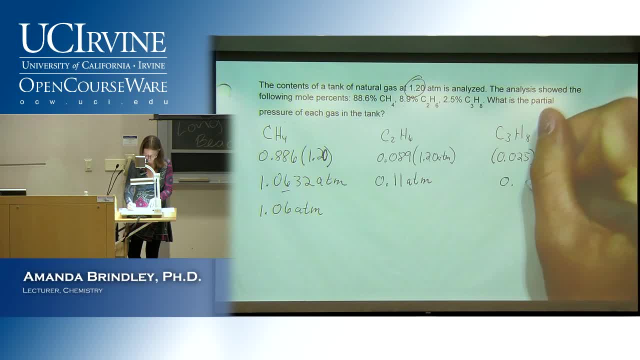 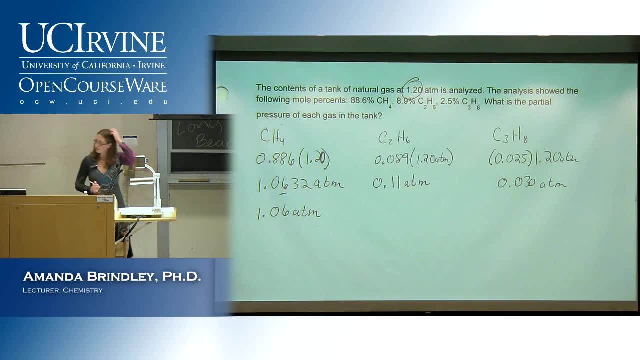 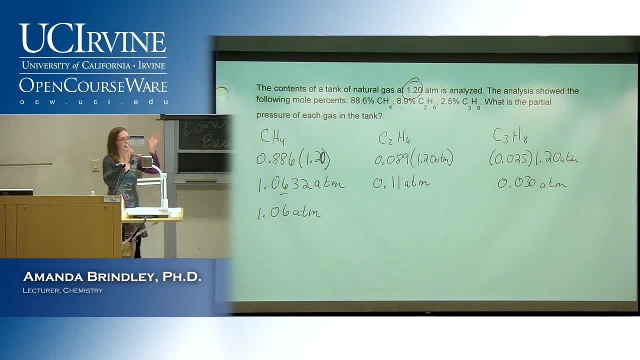 CH4. CH4., CH4., CH4. CH4.. Do you have to calculate anything? First of all, if let's say I ask that right from the beginning. I gave you this problem And you know how I write the exams, right? 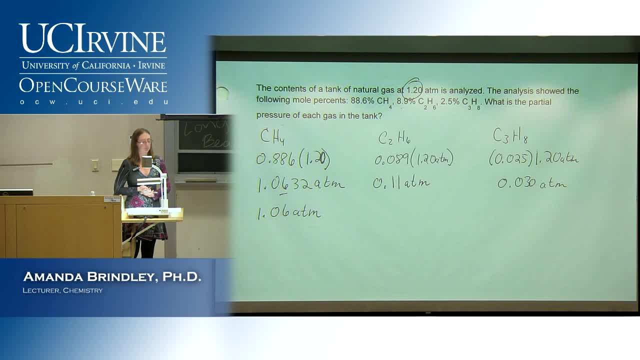 Lots of times there's multiple parts of the question in one thing And all I said is: you know, I wrote all of this out and I said: what is the mole fraction of each gas and what is the partial pressure of each gas? What would your mole fractions be? 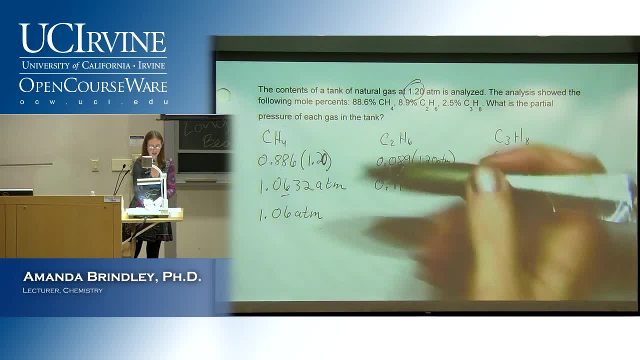 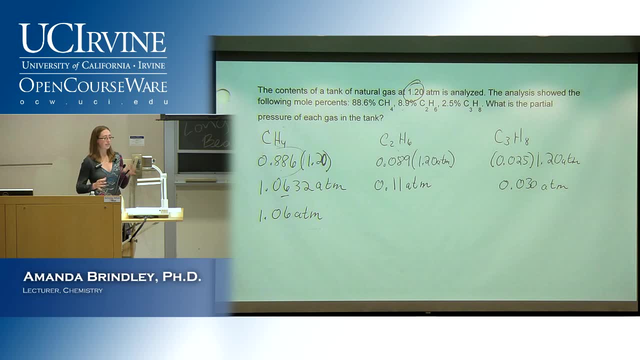 Yeah, it would be these right. In this one it would be the .886.. In this one, the .089.. In this one, the .025.. So if I give you, if I give you the percent, you just turn it into a decimal point and 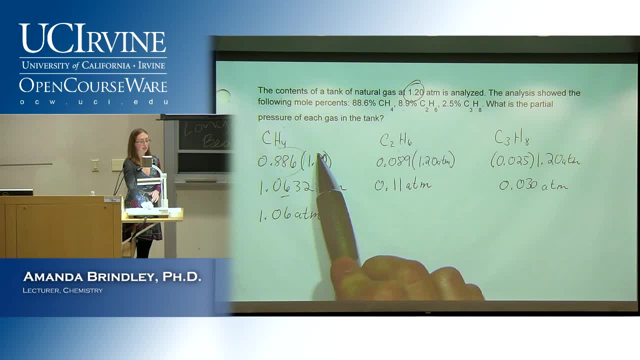 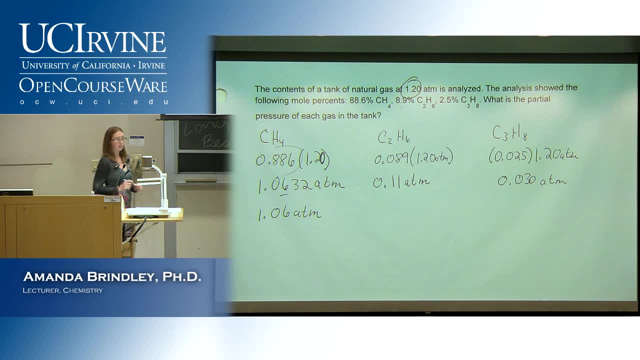 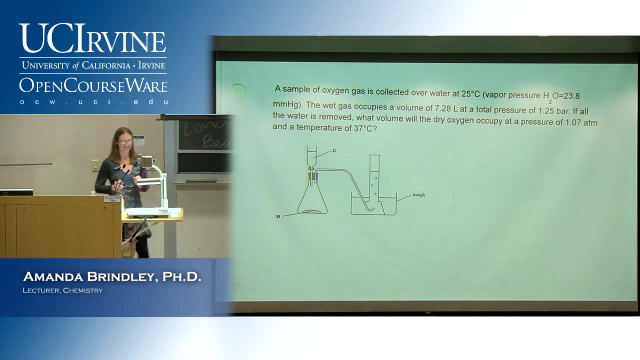 that's your mole fraction, right? That's why we multiplied this by this. We took our mole fraction and we multiplied by our total. OK, All right, ready for a much harder example. now You're supposed to be excited. no groans, be happy. 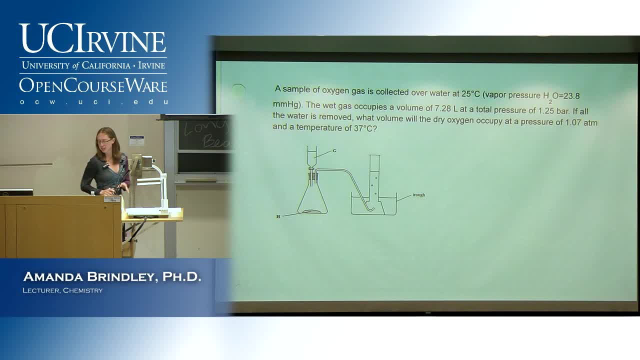 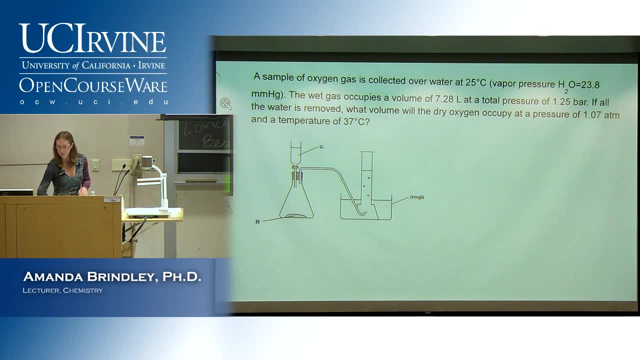 All right. so there's a little picture here which I think probably got added after the exam or after I had posted this, So let me zoom in a little bit, even though I'll probably end up having to zoom out- so you can see it. 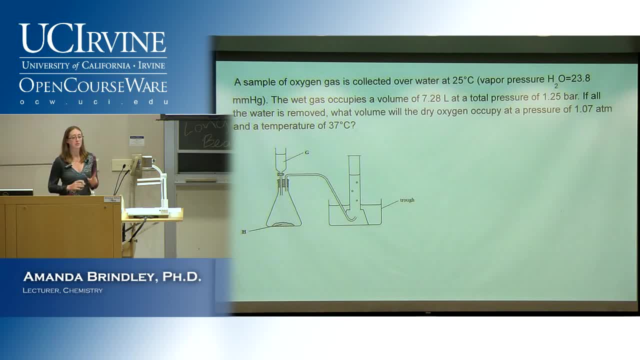 OK, this was because, when you know, this is a little bit of a confusing setup, but it's a very cool setup and something that you can do in lab and you can do, you know, probably not at home, but definitely in lab. 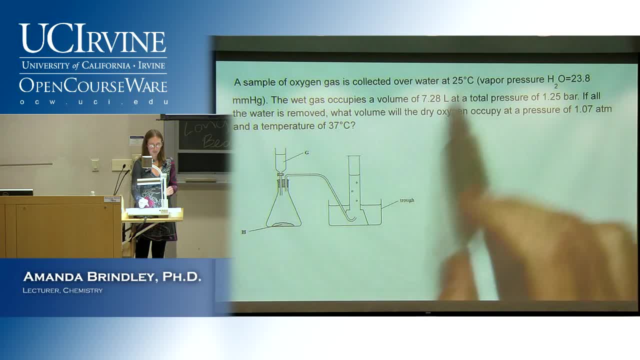 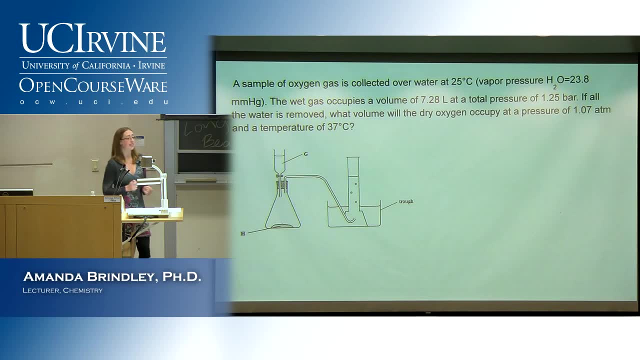 So we have a sample of oxygen gas collected over water. So what's happening? What's happening here is some sort of reaction is going on here, some sort of reaction that makes oxygen gas. So in this case there's a little beaker where something is going on. 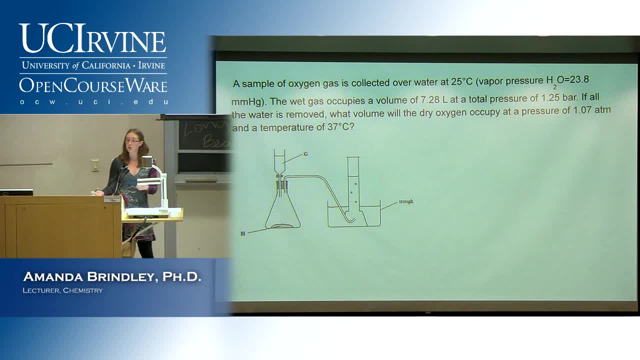 The other time this will happen is you can burn something and make CO2.. So this is a way of measuring how much of a gas comes off, a reaction, which is useful if you're trying to figure out something about how the reaction is happening. Maybe you want to know a percent yield, or you want to know something about a reaction. 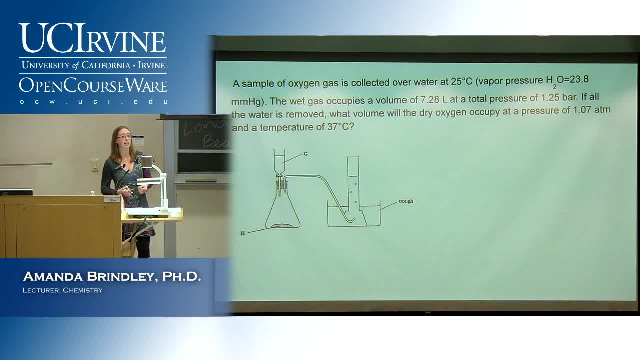 and you need to know what all your species are. You need to know how much product you get, How much product you get out of each one. Well, this is the one way that you can test for oxygen, or that you can measure oxygen, if it's the only gas that's evolved. 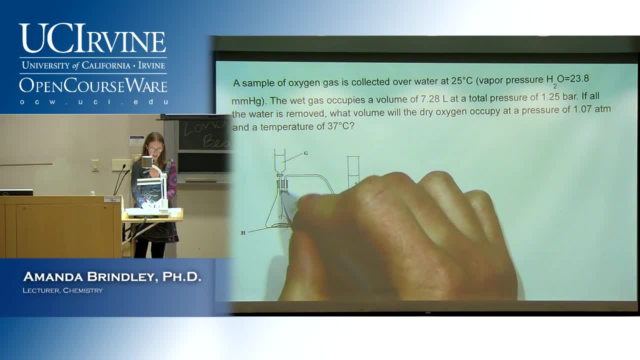 So what happens is you have something going on here. You have a reaction happening. Oxygen gas comes through here- It's the only place for it to really go- and then it bubbles up. So you have a tube that originally was completely filled with water. 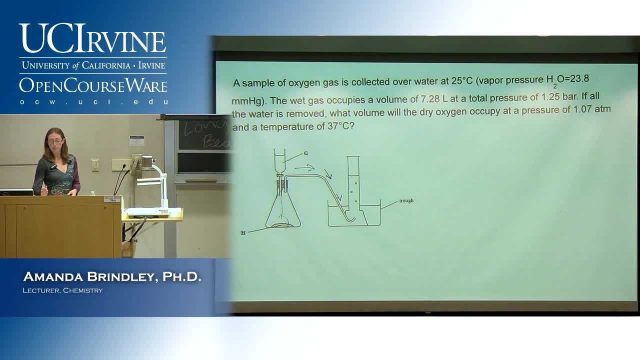 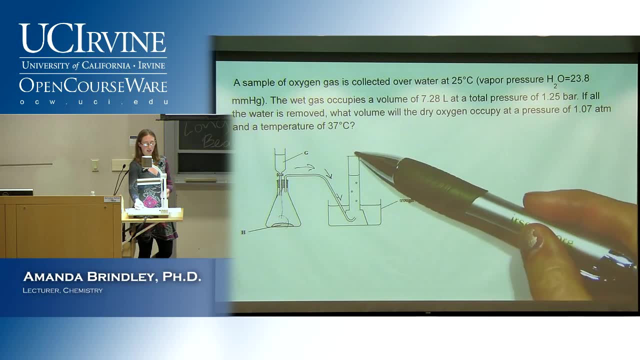 You have a tube completely submerged with water. You stick it into a beaker. a flat thing of water here, And then the only air in here or the only gas in here comes from this reaction, which will all be oxygen. So this is the way that this setup works. 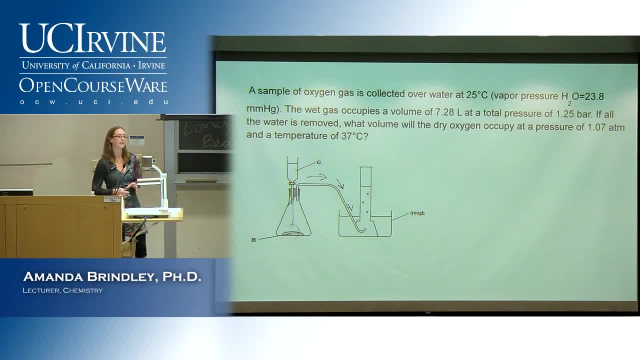 And this is: I don't think you guys do this in lab, unless it's been added in the last few years, but this is something that a lot of labs do. So what can you do with this if you have this and, let's say, you put it in a graduated cylinder? 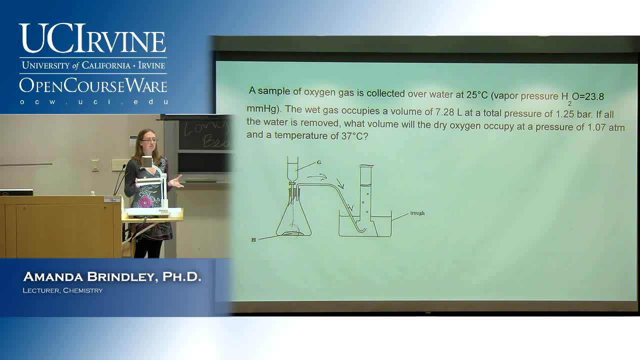 You can measure that volume right. Can you measure the temperature? Yeah, sure. So you know a lot of things about the system and you can measure how many moles of gas are in here, And that's what we're going to do in this problem. 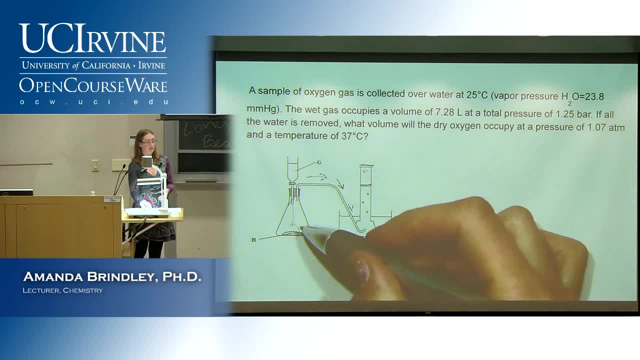 We're going to try to figure out how many moles of oxygen came off this reaction. So when we say it's collected over water, this is how they actually go about doing it. They have a cylinder filled with water. They put a tube in. 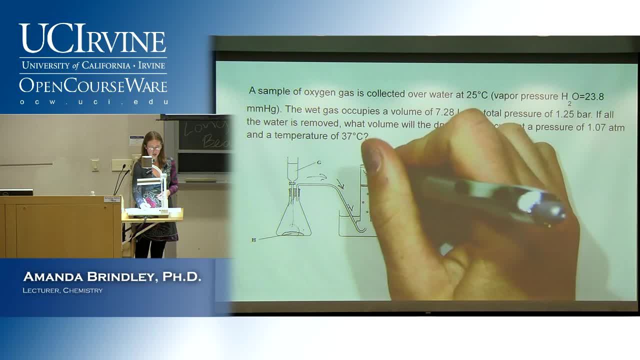 The gas bubbles through And then you can- as long as this is like some sort of gravity, Yeah, Sort of graduated system, you can see the volume of gas that you collect. So I say a wet gas. well, how can a gas be wet? 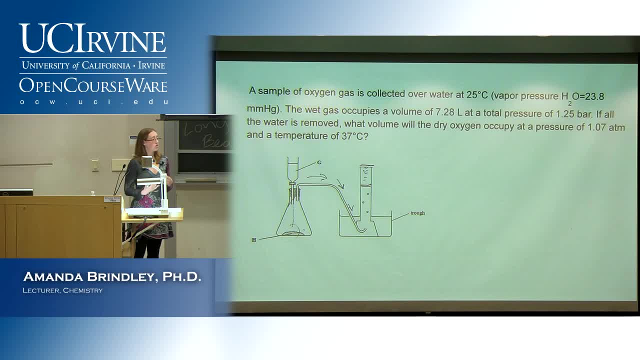 What that means is that it has water vapor in it. It's not pure. So if you take a- you know a tank of oxygen that you don't want any water in at all, they would have done something to take out the water vapor. 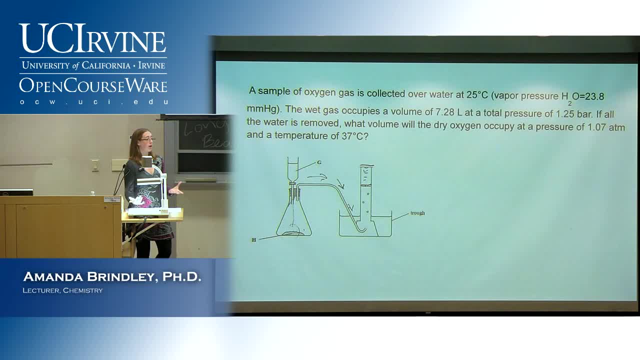 In this case it's sitting over top of water, right, We know that water evaporates. We know that water has a vapor pressure And if you put some water down here it's going to evaporate. And if you put a cap over it it's going to, you know, condense and evaporate and do its. 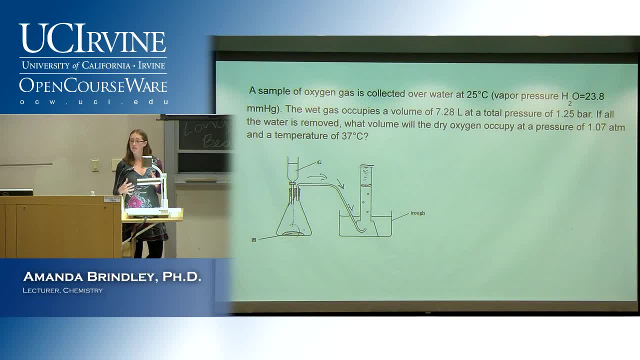 thing. So there's water vapor in here, So that's going to change the volume a little bit. So we have two things right: We have water vapor and we have the oxygen gas. So two things that we have to worry about. 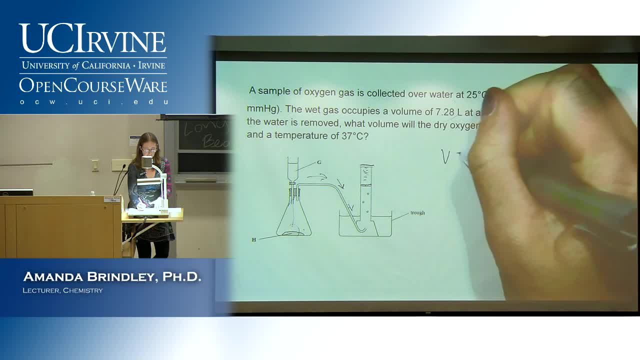 But those two combined have a volume of 7.28.. So that's our total volume. Okay, We have a pressure of 1.25 bar And that's our total pressure. If all the water is removed, what volume will the dry oxygen gas occupy at this whole new? 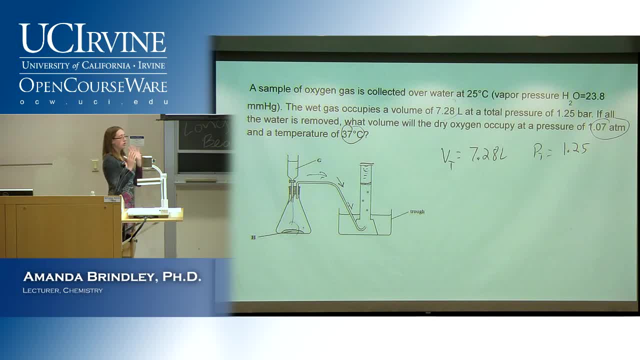 set of conditions. So we're taking what we just learned with Dalton's Law of Partial Pressures and we're going to combine it with what we did last class where we went through and did final and initial conditions. So a lot going on here. 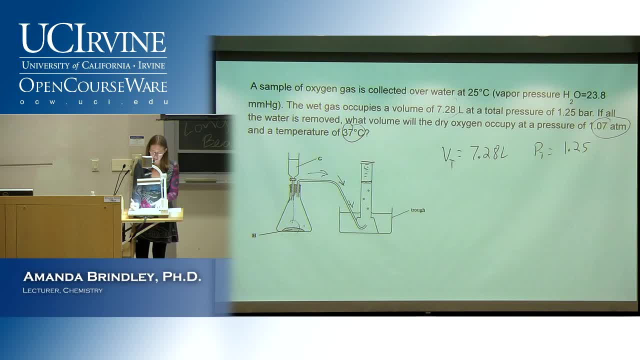 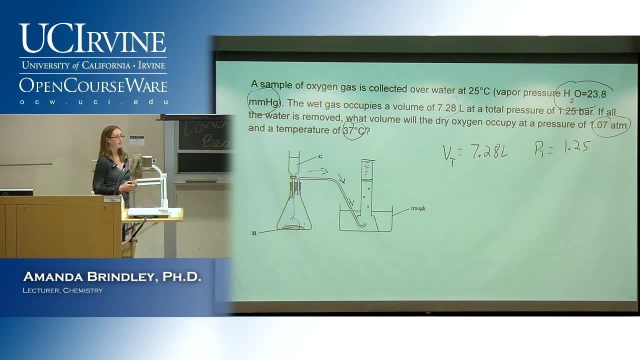 This is a tough question, Okay, So just to make life a little bit more fun, I also gave it to you in the wrong unit so that we could practice playing around with units. So this right here, that's water vapor, right? 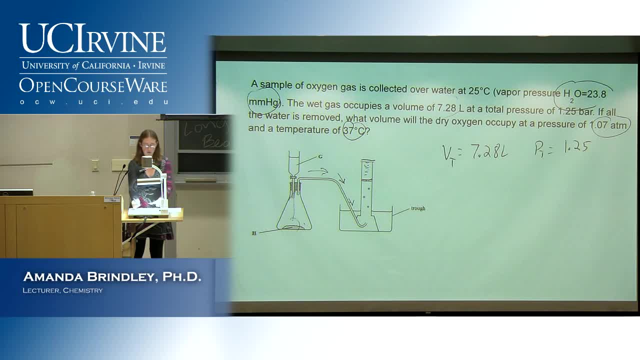 That's the pressure of the water. So we know that this pressure is going to be what the water is. So then, how do we go about finding the pressure of the oxygen, The initial pressure of the oxygen? Yeah, So let's write this out a different way. 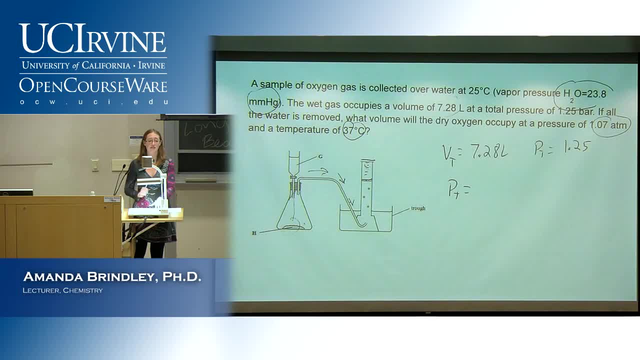 We know our pressure total has to be the pressure, the addition of all the gases that are in there. So what is in this little, what is in this beaker right here for gases, Oxygen. So we know the pressure of oxygen plus. 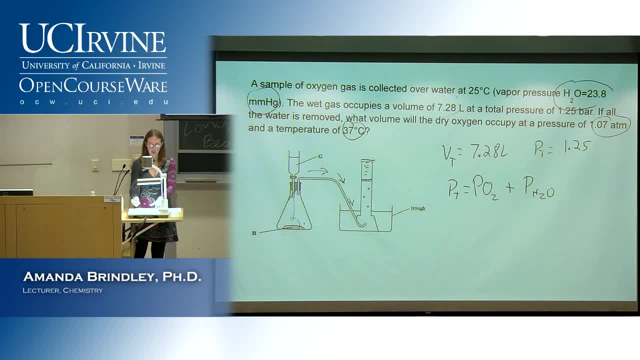 Yeah, Okay, Now we're getting somewhere right Because we have this, we know, we know our pressure total is 1.25 bar and we know our pressure of our water is 23.8 millimeters of mercury, So we can find our pressure of oxygen. 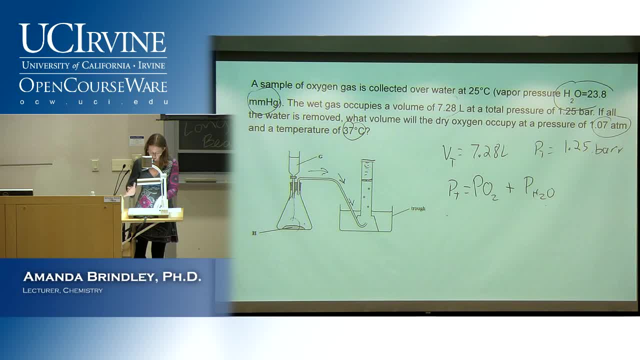 So we're definitely we're getting closer. So first we have to do some unit issues So you can really switch to pretty much any unit you want. here I happen to switch everything to millimeters of mercury, Sorry about that. That should be 1.25.. 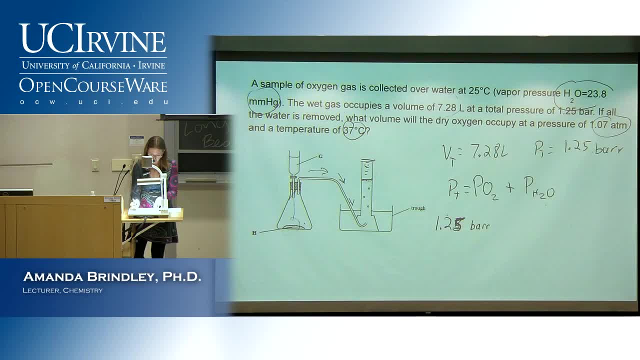 So we're going to take the 1.25 bar and I'm going to convert that into millimeters of mercury. Okay, You could convert it the other way if you wanted. And of course, all of these conversion factors are given to you on an exam, so don't spend. 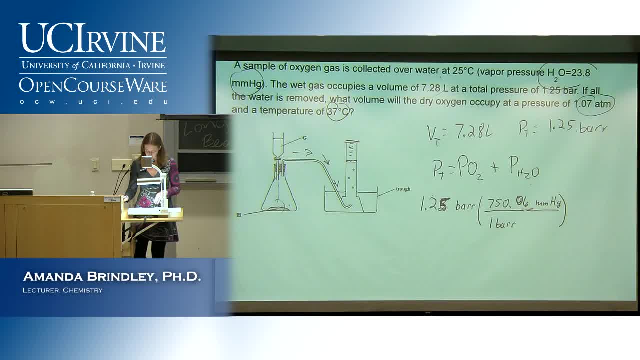 any time memorizing them, Okay, So now we have this and we can write down that value, And I'm going to have to zoom out a little bit now that you guys have had some time to look at the picture. So this is our total pressure. 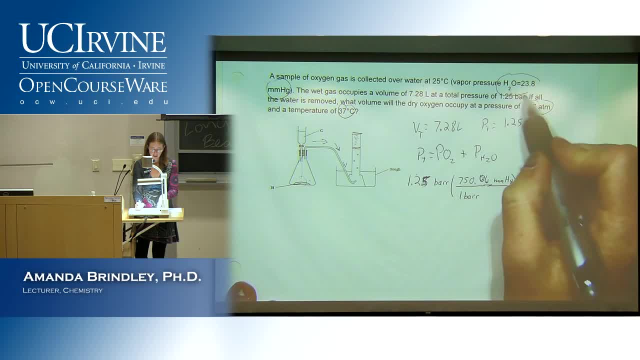 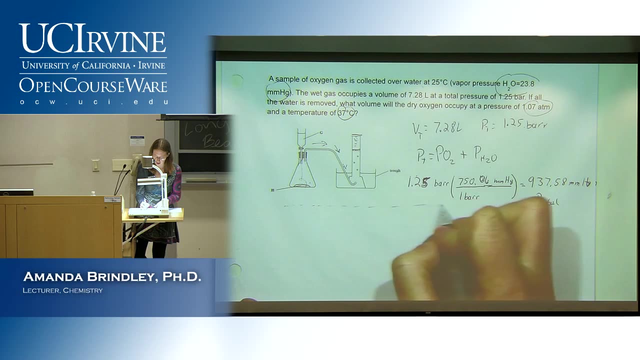 Now I'm going to fill this in. Okay, So that, once again, is going to be our total pressure. Okay, So now we can start filling in some values. We need to know the pressure of oxygen. So just for the cleanliness of work purposes, I'm going to draw a line here. 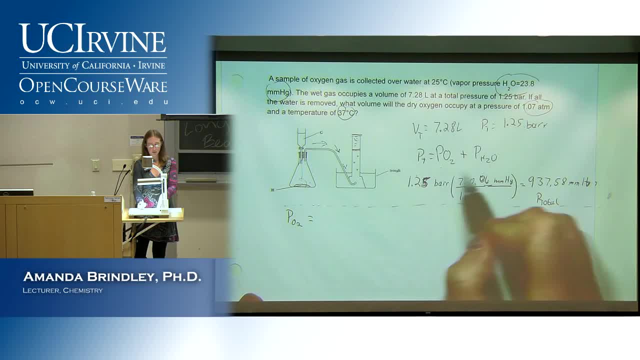 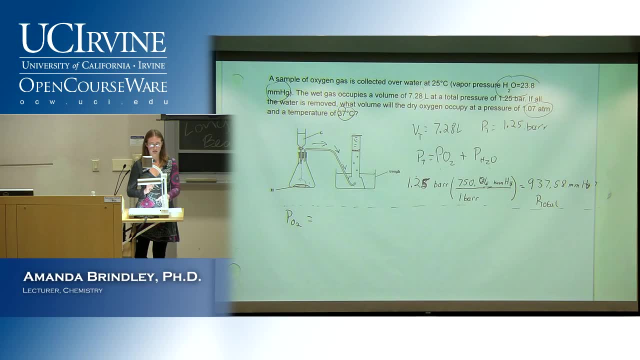 So we need to know a pressure of oxygen And we can get that through this equation right. We know that our total pressure is only equal to the pressure of those two gases. Okay, So how do we get our pressure of oxygen? 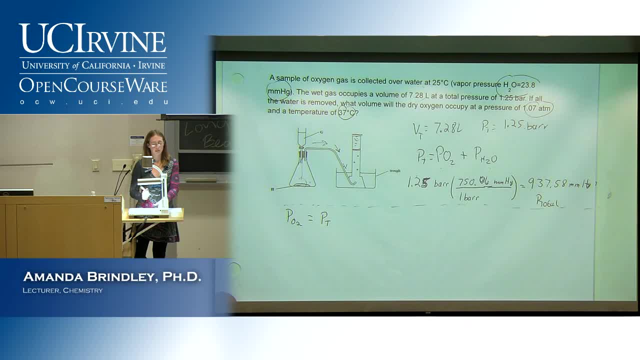 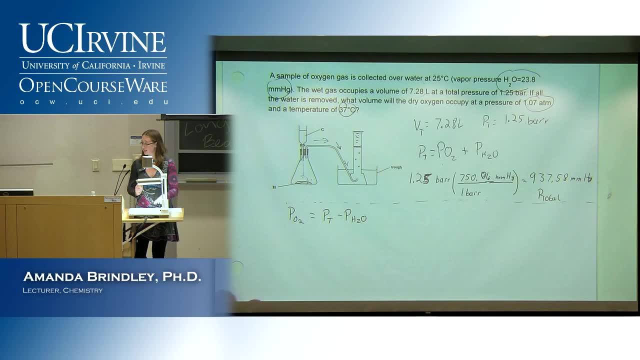 PT. and then what Do we add? our pressure of water? Good, we subtract it, And so we get that. Now, since we've switched our units around for this purpose, we can go ahead and fill in Now something that's worth kind of doing up here, because we're going to be doing a. 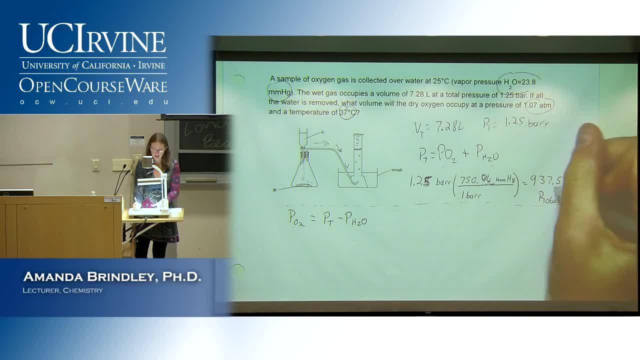 lot of calculations with things that we calculated is to watch your sig figs. start using your underline method, where you just underline the last significant one so you can keep track of what's happening here. It's way too much work to try to, you know, trace it through otherwise. 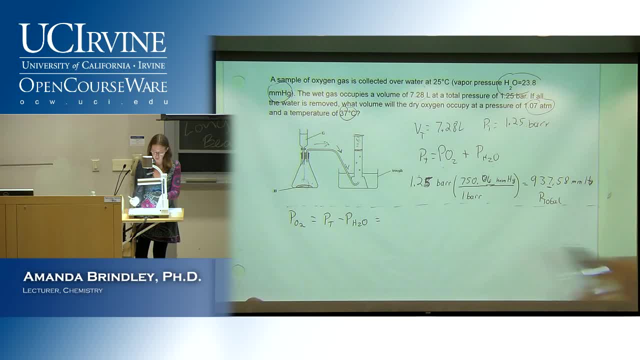 So we'll go through, We'll fill in our pressure of each one, because it's a bad idea to round every single time you fill in. To be honest, I tend to just save everything in my calculator, Okay, And then, for the sake of units, put that. 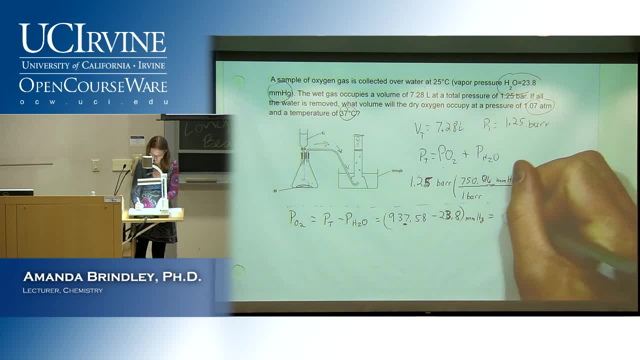 And so we can get our answer. Now we have to pay attention to sig figs a little bit here. What are we going to round to? So I'm hearing three and I'm hearing tenths. So if this was multiplication and division, you're right with three. right, because there's. 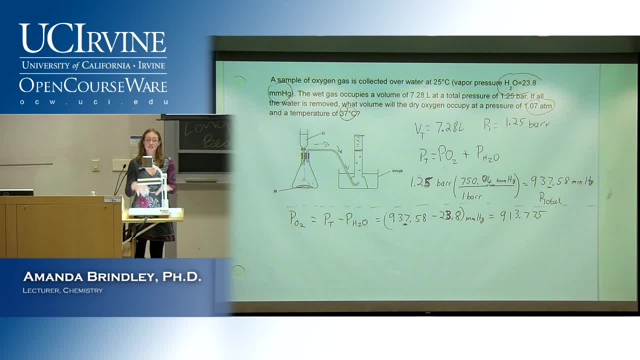 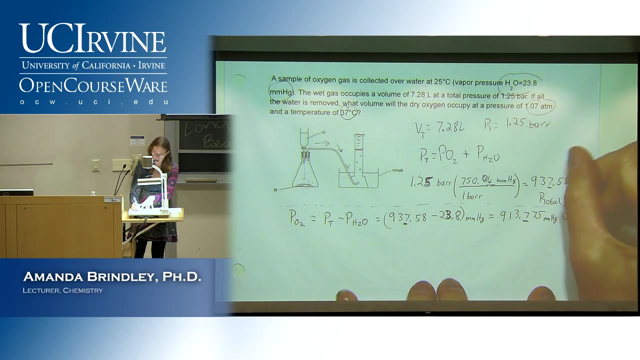 three. The number is three sig figs. But this isn't multiplication and division, it's subtraction. So we round to our lowest digit, So our tenths place, So we round to that Okay, So that is our pressure of oxygen. 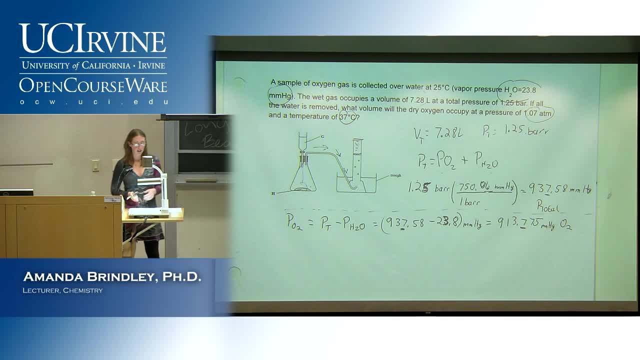 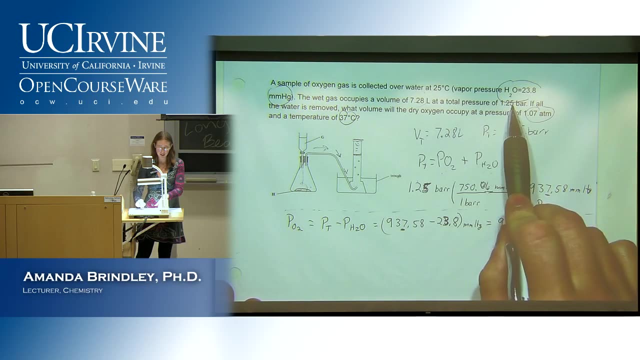 Are we done? No, right? No, So this is our pressure of oxygen. under what conditions? These right, This is our condition at 25 degrees, and this pressure, or, excuse me, the 1.25 pressure, total in that volume. 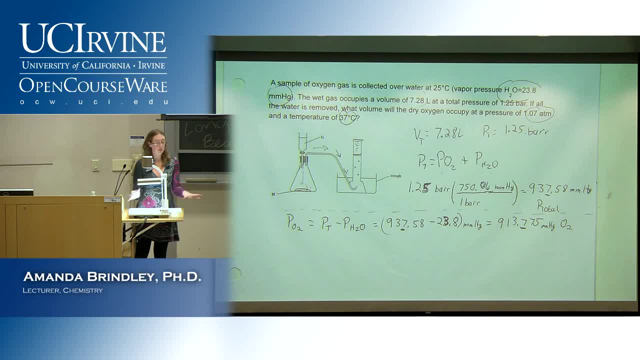 That's not what I asked you. That would have been too nice, right? I said now we're going to change everything because in reality, if you were going to do this, probably you would change the situation. Probably you would end up, in order to dry the gas, you would have to do something to. 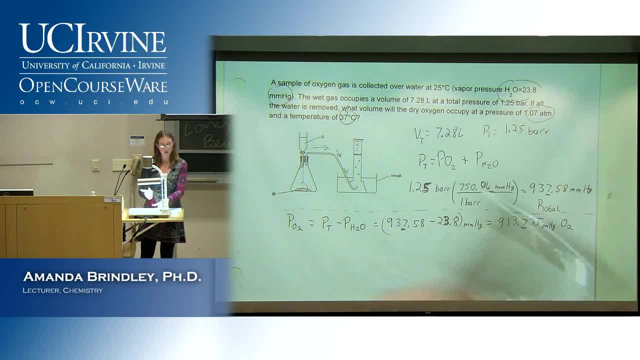 it, And so that's going to change your conditions around a little bit. So this is what we're going to do. We're going to do the exact same thing that we did last class. So this is going back to the material then. 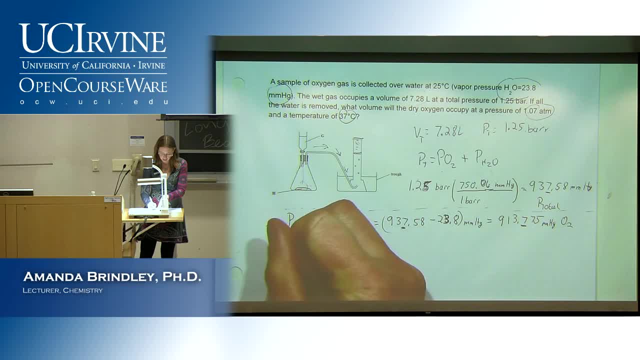 And we always started from this equation, right, Because we figured: well, we start with everything changing and then we just cross off whatever doesn't change. So we start from this one more time. Now- the nice part about this- do we have to worry about the fact that I'm in millimeters? 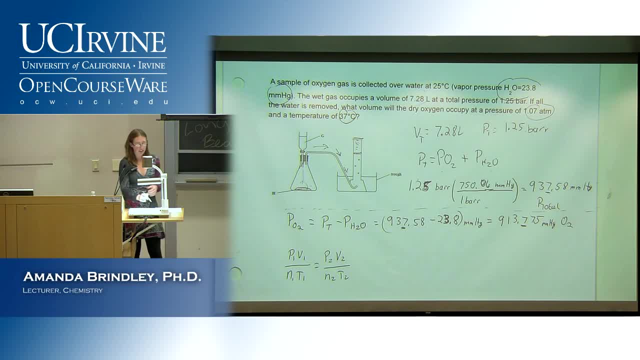 of mercury. No right, Because whatever I plug in here, that's just what's going to come out for my final pressure. So that's not a big deal, OK, Or, excuse me, we do actually have to worry a little bit. 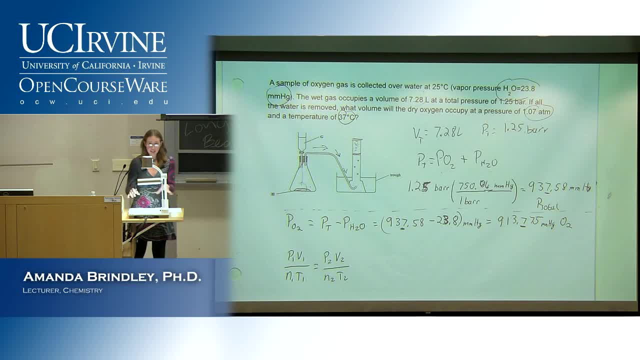 We have to convert from one or the other. So it doesn't matter what unit we put it in. It doesn't have to be in atmospheres, it doesn't have to be in millimeters of mercury, but it's got to be in the same thing. 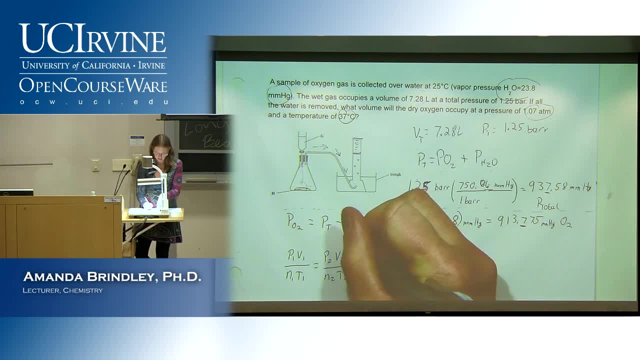 Now our volume. So let's go through and convert all of this. We're solving for what variable? V2.. V2. OK, So we'll fill everything else in. So our P1 comes from here right Now. I think in this case I converted everything to millimeters of mercury again. 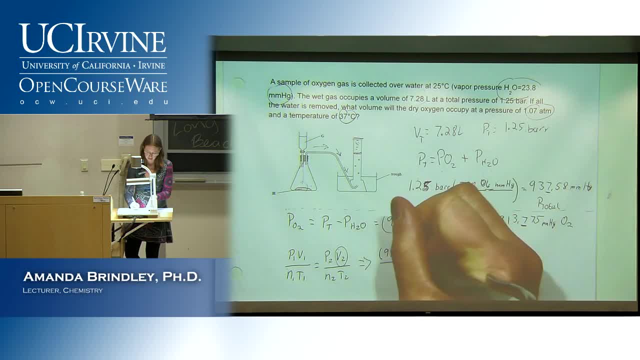 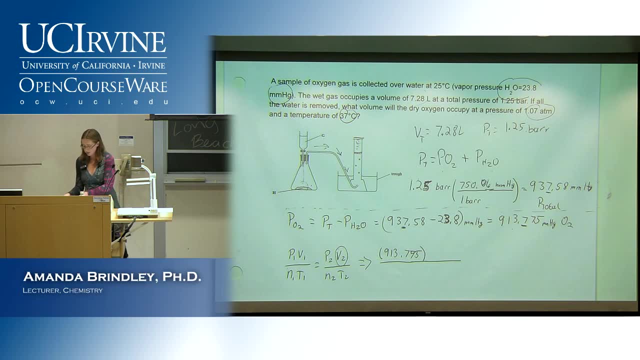 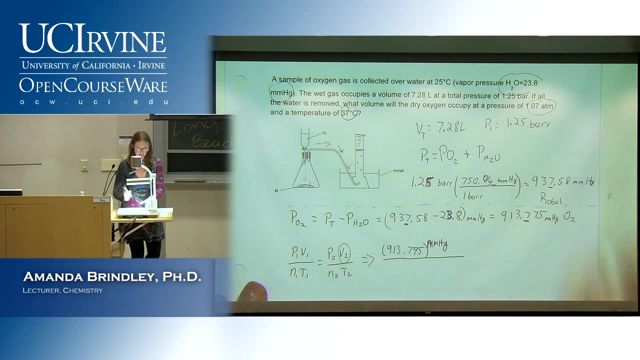 I was apparently in a millimeters of mercury day that day. For the sake of room, I'm going to be a little bit lazy about writing units. Perhaps We'll see. So this is in millimeters of mercury. Now our V2, or our V1,? what is our V1?? 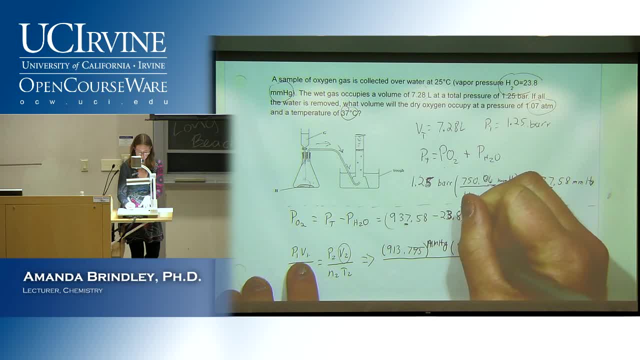 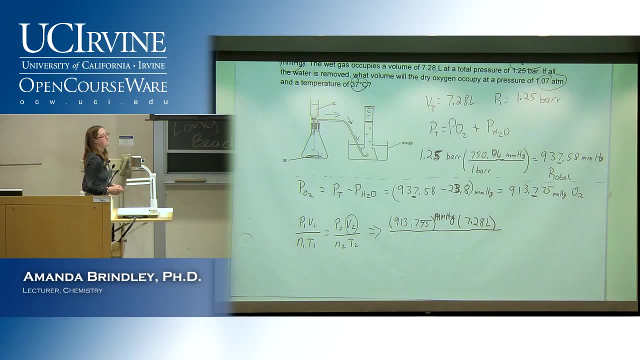 That's that right. So we go ahead and rewrite that in. I've decided in hindsight not to be lazy about units. it's too complicated of a problem. So that's our V1.. OK, So now our N1.. Do we have to worry about N here? 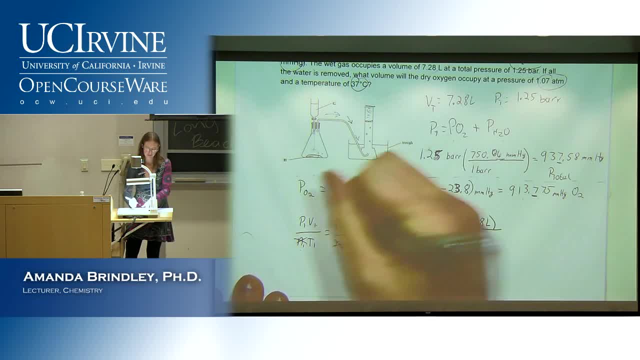 No, That gets cancelled out. So we don't have N. but we don't need to worry about N because we're not changing it. So that goes away. So our T1. Is our T changing? Definitely? So I'm just going to fill in 25 here, then, right? 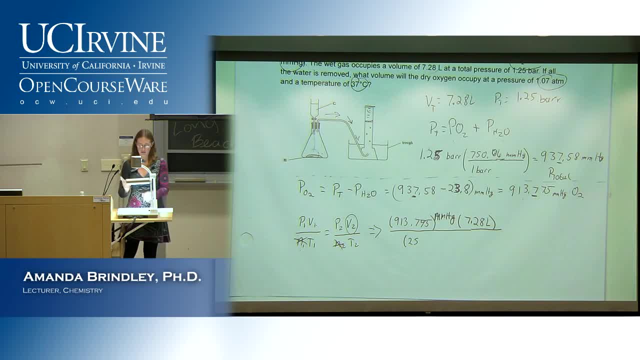 No, No right. What do you have to do, Kelvin? Don't forget that It's really the most painful mistake to have to grade on an exam, Because we know that you know the difference, But if you forget, it's wrong. 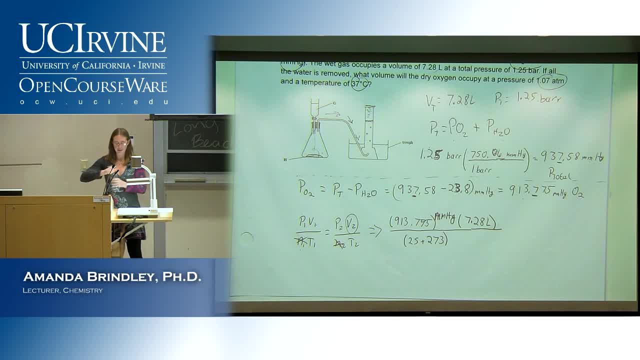 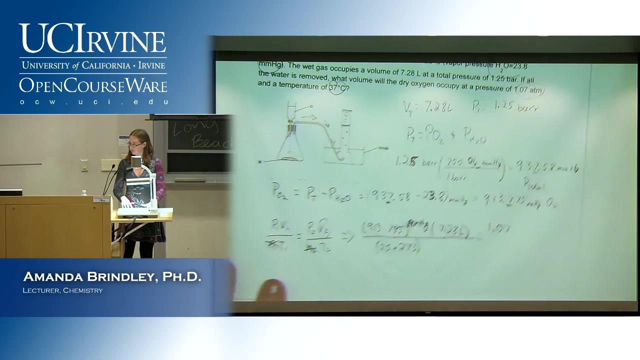 So excuse me one moment. OK. Next part then P2.. Do we know P2?? Sure, It's given. So I'm just going to fill in 1.07 and go about my merry way, right, No, OK. 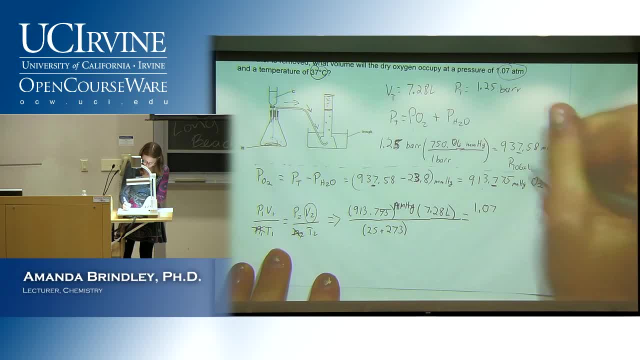 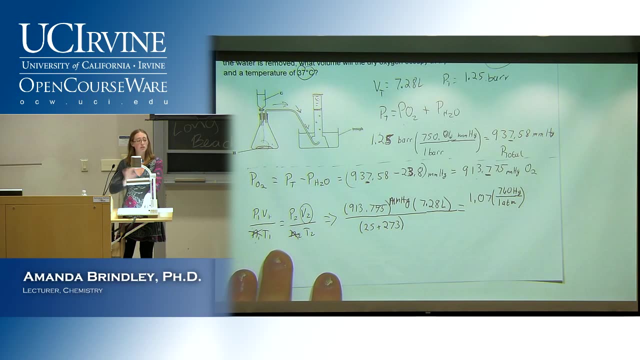 So we need to go ahead and we need to convert this. So that's an ATM. So we fill down ATM here, We fill in our conversion factor up here- You can always do this on a different sheet if you want to- and then fill it in whichever. 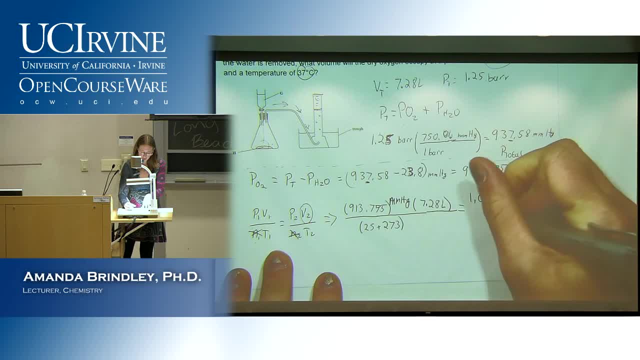 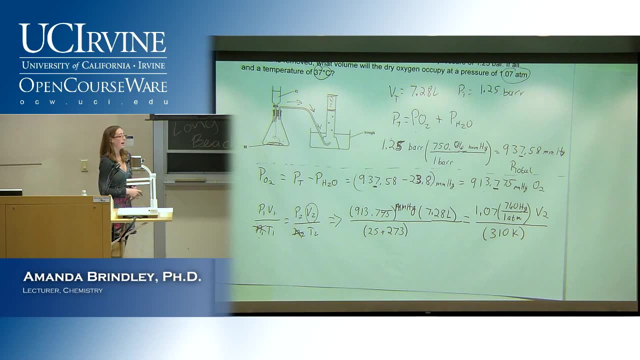 way you prefer. We fill in V2. And we fill in our final temperature. OK, So once we go through all of that and we do the algebra- which I'm not going to write out the algebra because, quite honestly, the easiest way is to just do it inside your calculator- 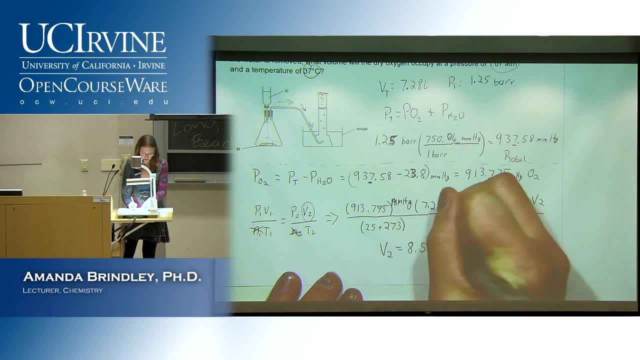 We have V2 is equal to 8.50 liters. Now let's check our sig figs on this last part. So We know that this let's just write in 290, so I'm going to actually just it's not wrong. 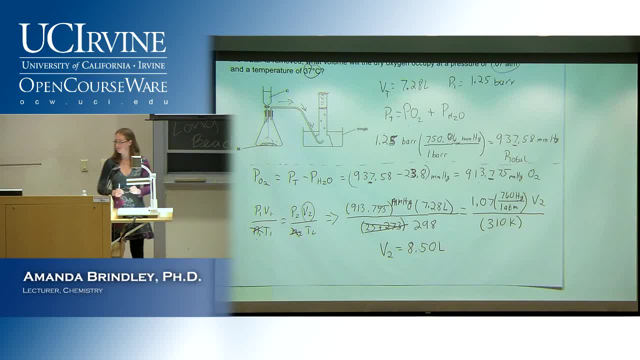 but I'm going to cross it off and write 298 for the sake of going through and doing the sig figs, because we know we're going to be at our ones digits here. Now, what's our sig figs here? We took 37 and we added it to 273.. 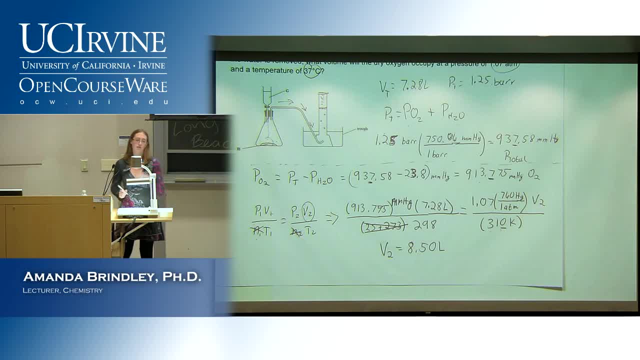 So is this really two sig figs? No, It's really three sig figs. OK, So watch out for sig figs in those types of situations, OK, So now we have how many sig figs here? Four. Three sig figs here, three sig figs here, three. this is actually three, by definition. 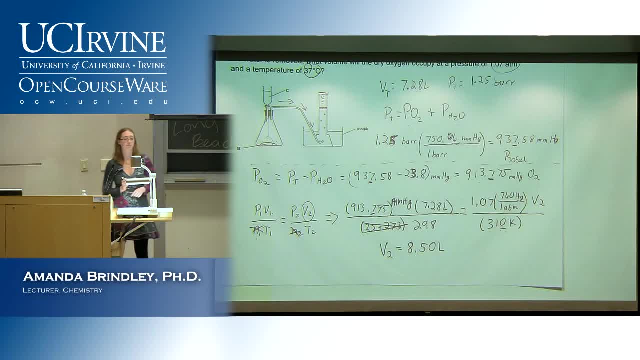 it's three and three, So we need to have three down here. So I'm going to put a little underline there too. All right, OK. So questions on that very long, complicated problem. This is one of those problems you probably are going to have to really get go through. 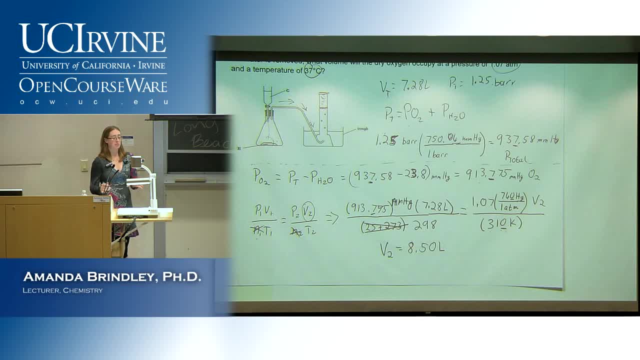 and do looking at the notes. do not looking at the notes, but constantly referring to them off and on for help and then maybe do again on your own. you know, three or four times before you really get it. It's long and complicated, but it's really just combining a bunch of things that we know. 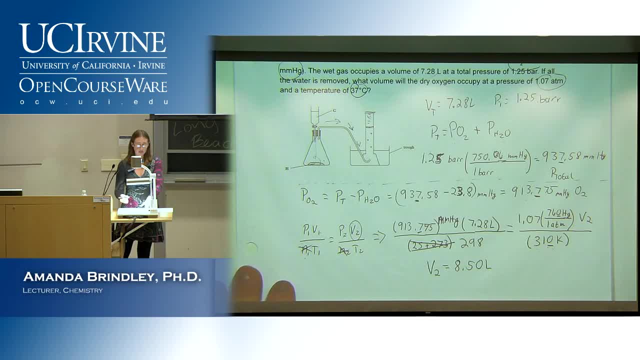 with one new thing. right, I gave you this new experimental setup, but we know that whatever that oxygen is, whatever that little volume is, we're going to have to do it again. OK, So what that little volume is is just our two pressures added together. 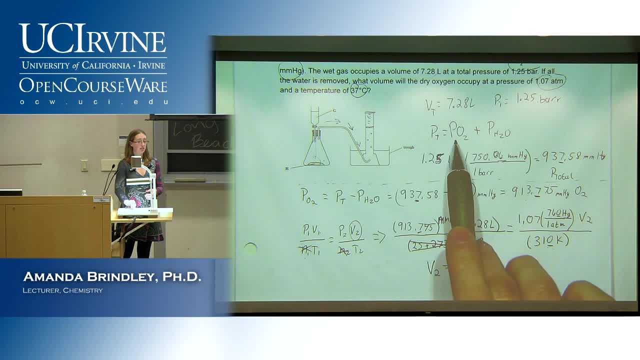 We know that. then if we want to find our pressure of oxygen after last class, last five minutes, we know that we can just subtract it from the total, because there's only two components, right, It's only water and oxygen. So we subtract that to find our pressure of oxygen. 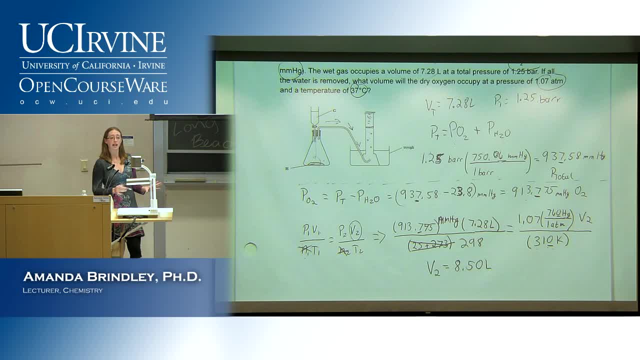 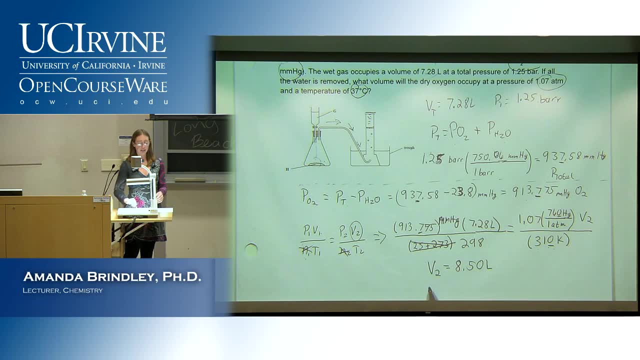 Now we're back to what we did for the whole first class, or the whole first half of class, last time and we said: OK, well, we have initial set of conditions and we have a final set of conditions. Let's solve for the unknown. 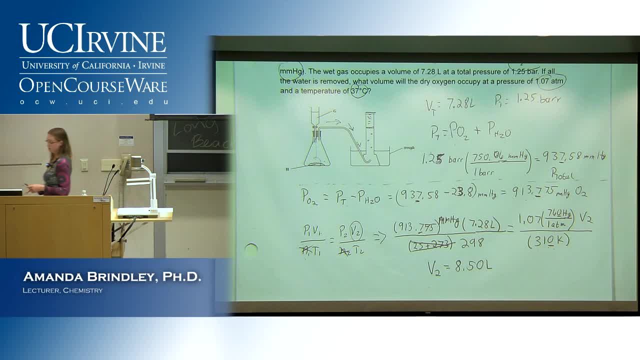 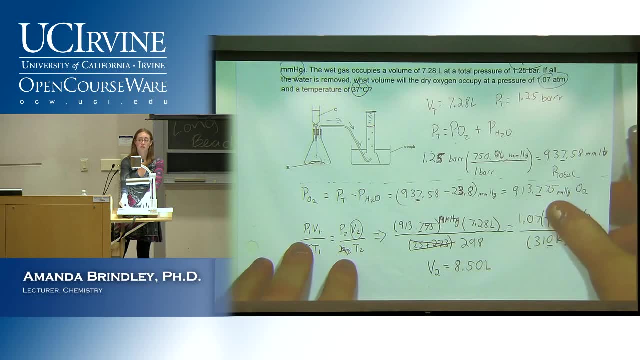 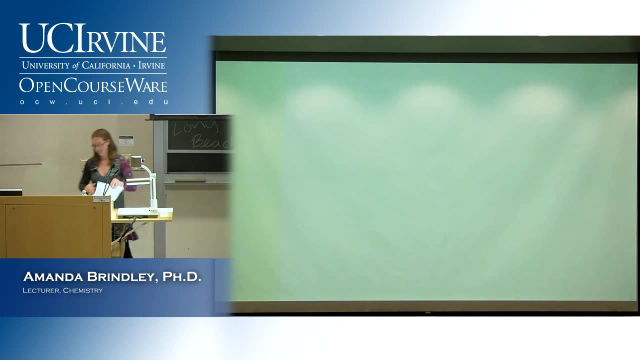 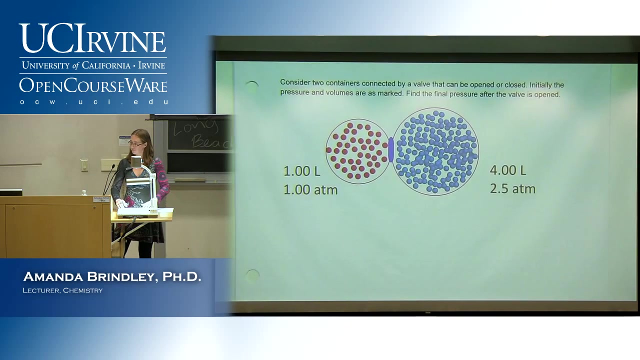 All right. OK, Any questions on that before I move on. You may be a little too lost for questions yet. That's fine. OK, We can revisit that one at a review session or something. All right, next one: All right. 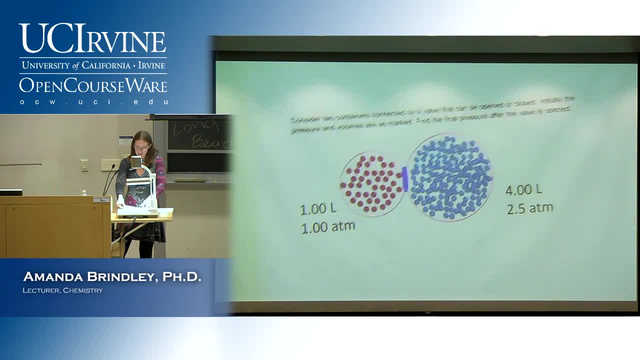 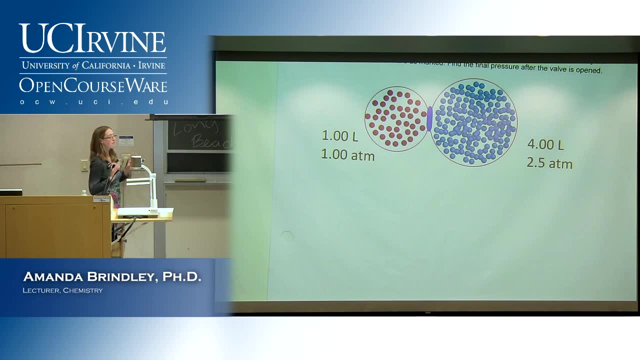 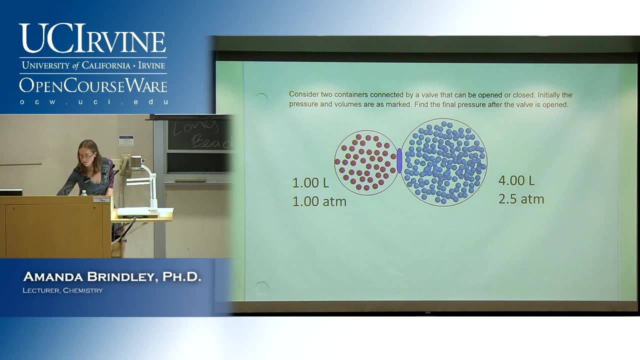 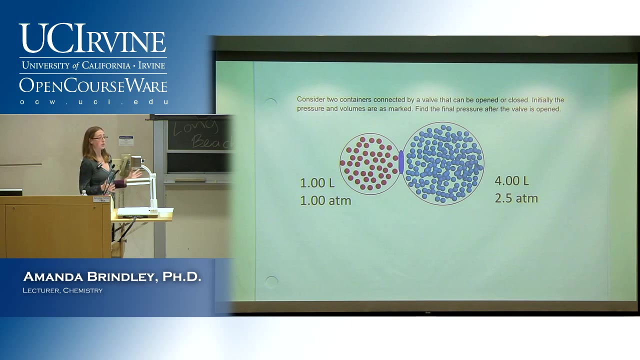 So we have two containers connected by a valve that can be opened. Initially, the pressure and volumes are as marked. Find the final pressures after the valve is opened. OK, So this could theoretically be a really complicated problem, But luckily Dalton's law makes it simple for us, which is really nice. 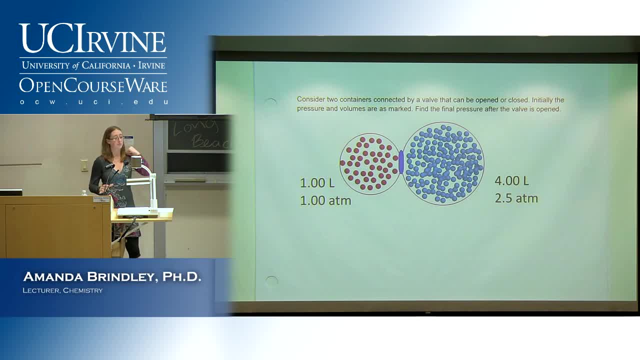 So we can treat this as two completely separate problems. What we're going to do is we're going to pretend that we open this valve and we that there's nothing here, that there's no gas here, that it's just a vacuum, and we let the pink come. 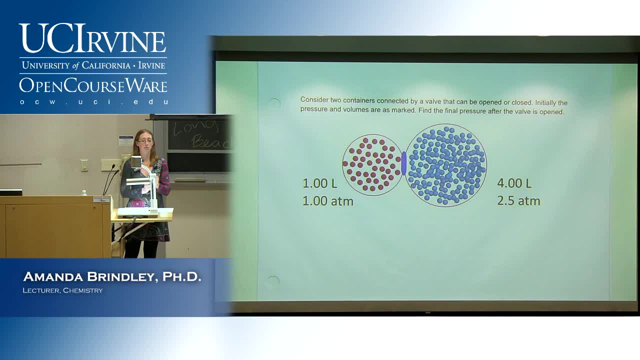 into here and equilibrate. We're going to pretend that on one half of the problem. Then for the second half of the problem we're going to go ahead and pretend that this goes into here, That this goes into a completely empty container over here. 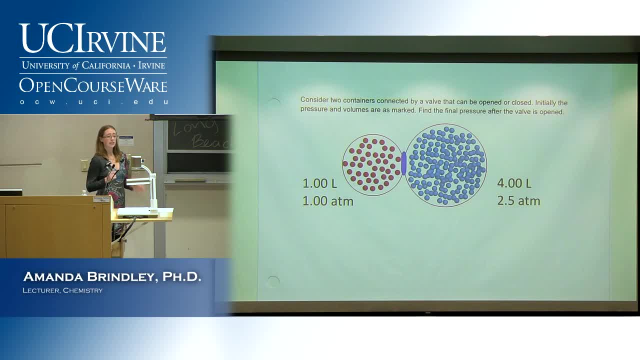 And that's going to be our second half of the problem. What that's going to wind up doing is giving us the partial pressures. So if we have the partial pressure of each gas, how do we find the final one? Yeah, we just add it together. 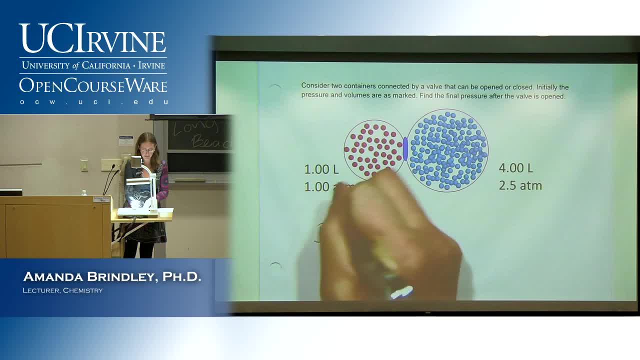 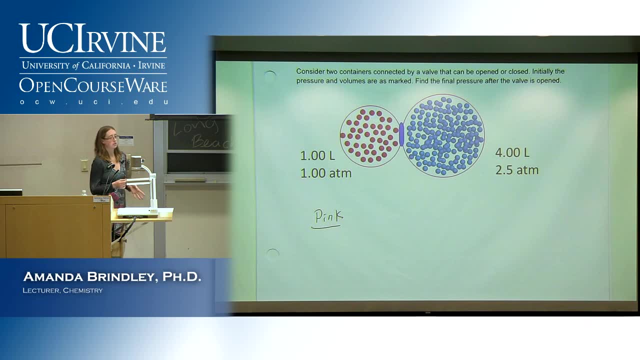 So let's go ahead and do that. So let's start with the pink side. So what all is changing here? Did I say anything about the temperature? No, Let's assume it's constant. Is the moles changing? What do we think? 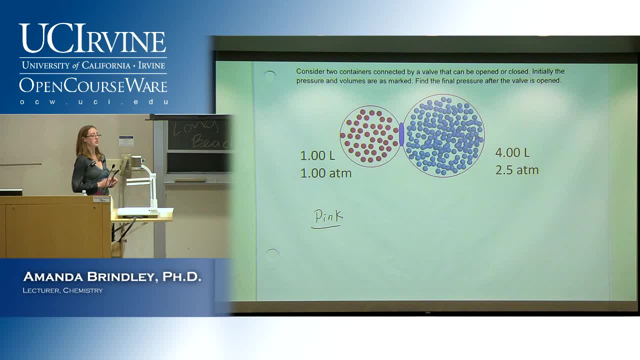 Do everyone? does everyone agree? Mostly because this is a tricky question. So they're right, but you know coral answers are good, right? It lets me know if you're understanding things. So why isn't the moles going to change? 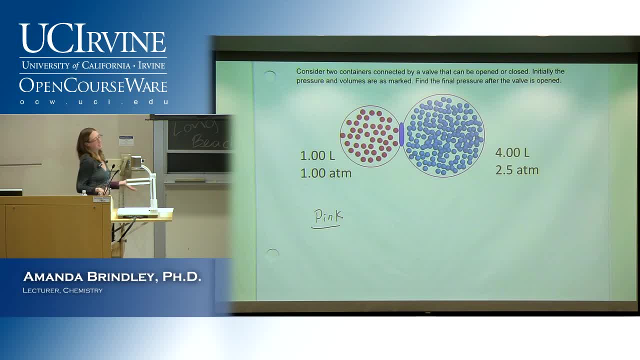 We're combining the pink and the blue, right, Yeah, but we're not talking about the blue right now. Exactly, We're not talking about the blue, so we don't care. All we care about is the pink going to change, And it's not. 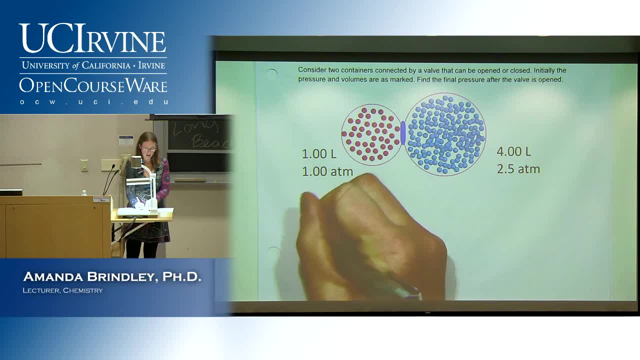 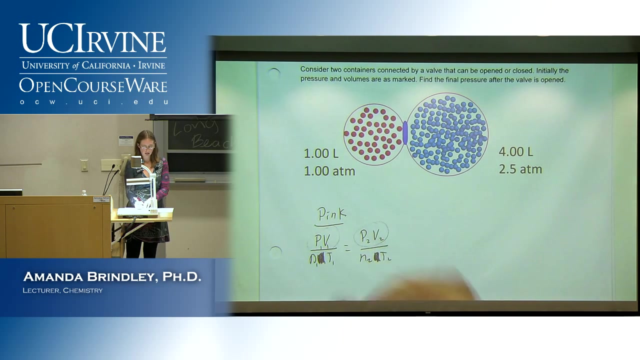 We're not going to take any away, We're not going to add any, So let's take away those R's. those aren't necessary, OK, So what do we have to worry about? changing then? Just P and V, So it becomes P1V1?. 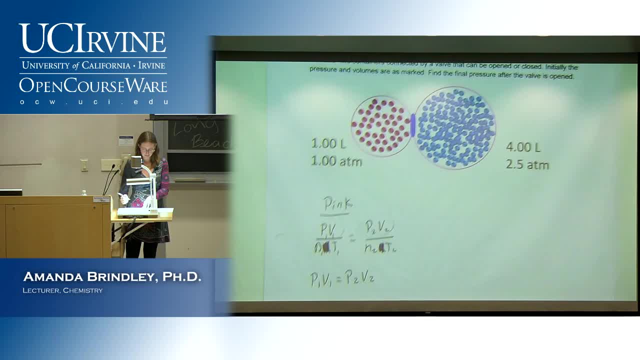 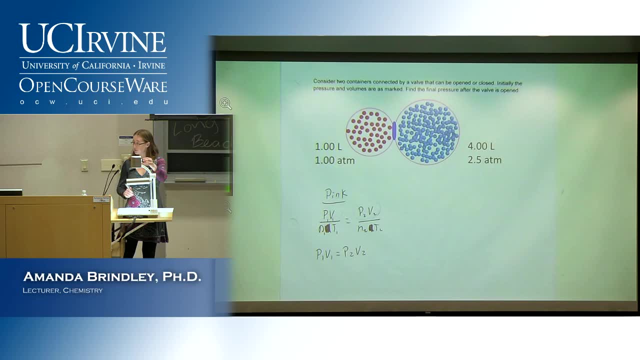 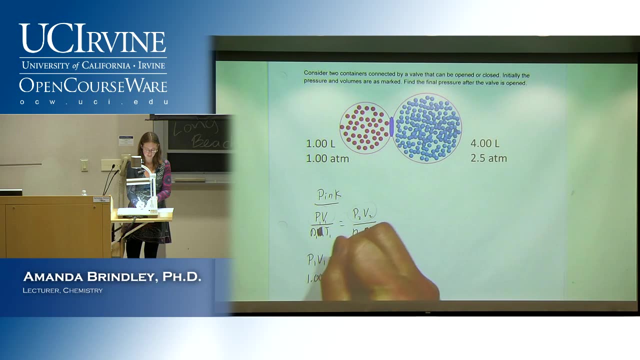 Yeah, Equals P2V2.. All right, So now we just fill in some numbers. So our P1 and our V1 are right here. Now. P2 is what we're solving for What is our V2?? Is it 4 liters? 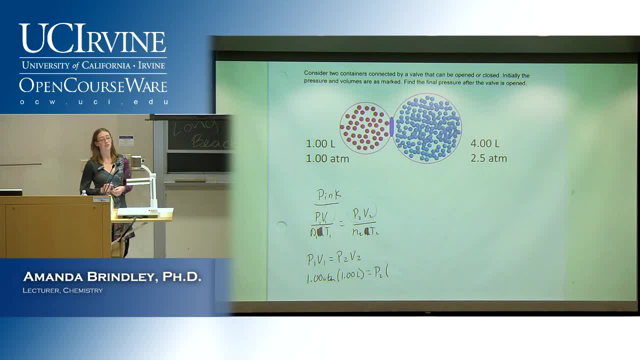 No, What is it? 5.? It's 5 liters, right, Because it's total. We're adding it together. We're saying this pink one can just spread out over the whole space and nothing in its way. That's kind of what we're pretending. 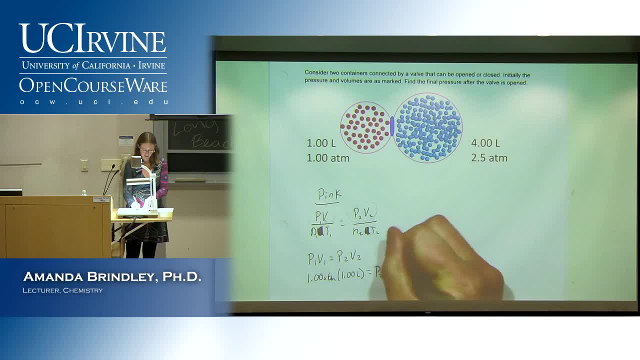 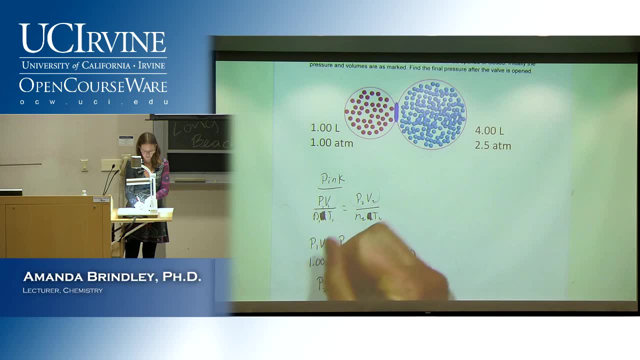 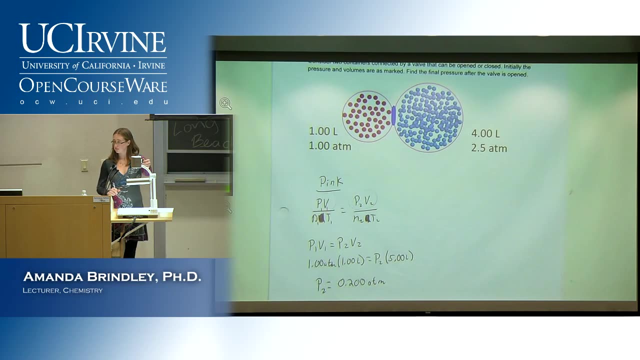 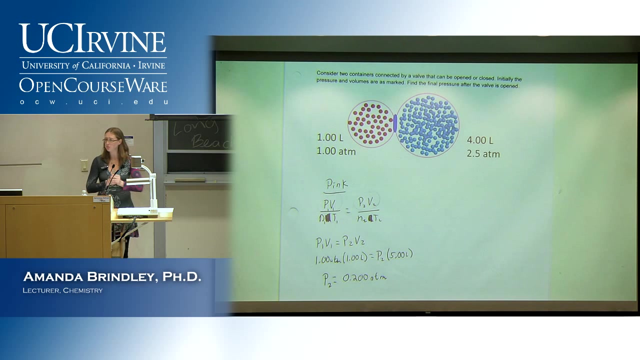 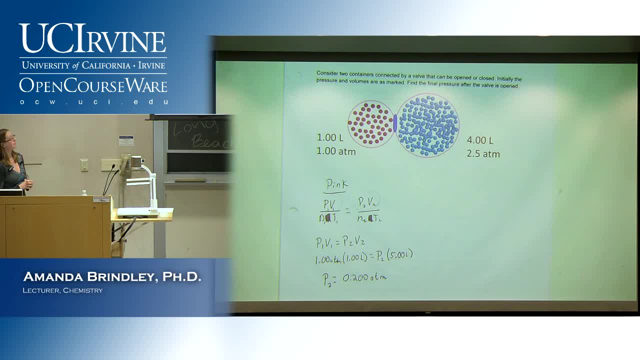 So take like a minute or so and do it, See if you can get the right answer, And then, if you can figure it out, find the total pressure as well. Oh yeah, Um, why is there already a pressure right next to the blue? 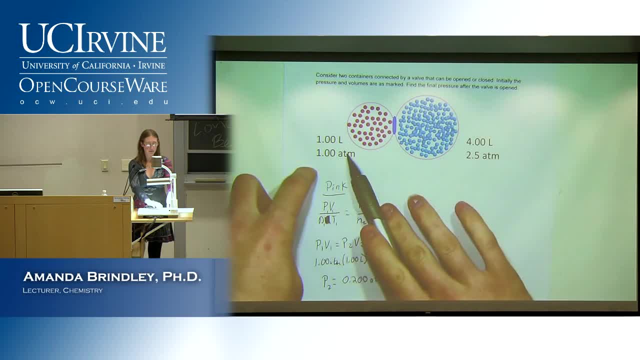 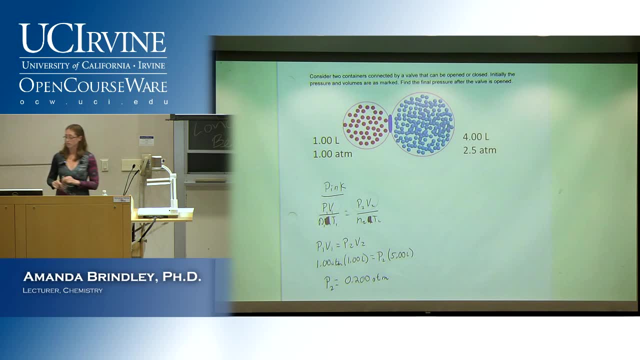 So these are the initial values. OK, the initial values of the pink and the initial values of the blue. All right, I'll give you 20 more seconds. You can talk to your neighbors, it's fine. I have like 10 more seconds to see if you have the same thing. 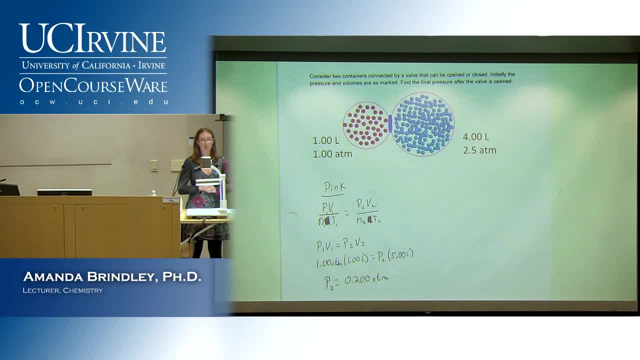 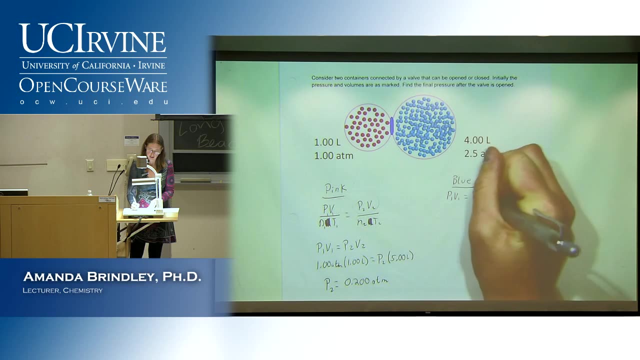 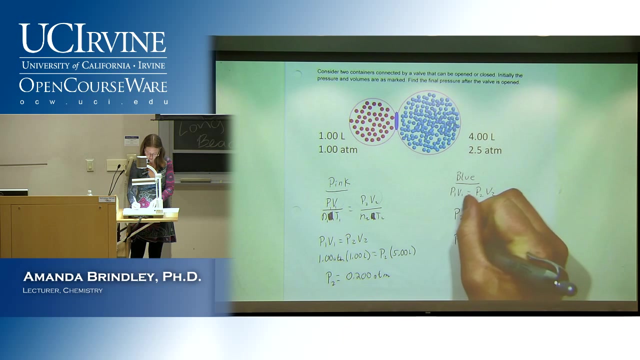 OK, what did you get for a pressure for the blue one? Do you guys agree? Two, Yeah. So I'm going to do this one solving for variables first. OK, This one's final is 5 liters as well. right, don't forget to add them up. 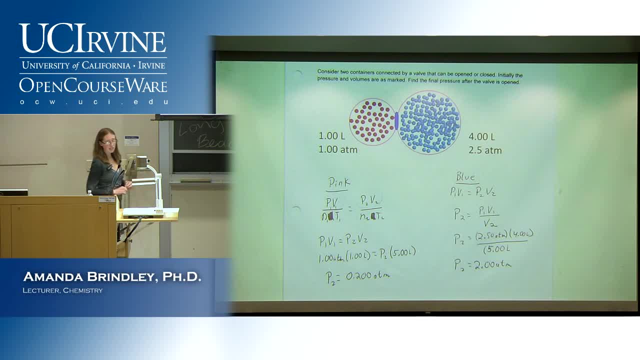 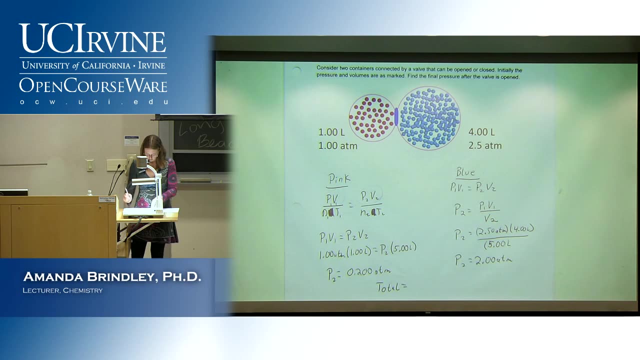 OK, so that gives us our partial pressures. So in this case, I just told you to find the final pressure, but the easiest way to do it is to go through and solve for the partial pressures. There are actually other ways to do it as well, but 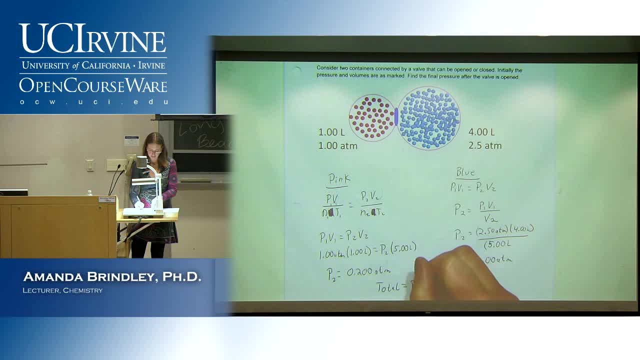 So let's go ahead and add these up, OK, So we get 2.20 at this point And we have a 2.20 in this period. We just have to keep going with this one, OK, so 10 times 4.. OK, 3., 5., 4., 5., 6., 6., 7., 7., 8., 8., 9., 10., 11., 11., 12., 12., 14.. 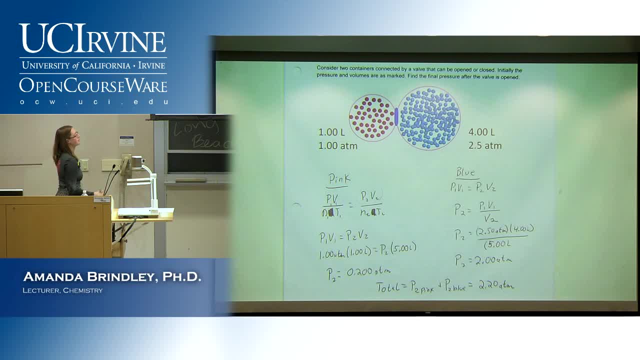 15. 15. 12. 12. 14.. I know I did the hard one first and then the easy one, but keep you on your toes. The next one. however, we're going to go back to hard. Really, I just needed to give you guys a little bit of a breather between the two hard ones. 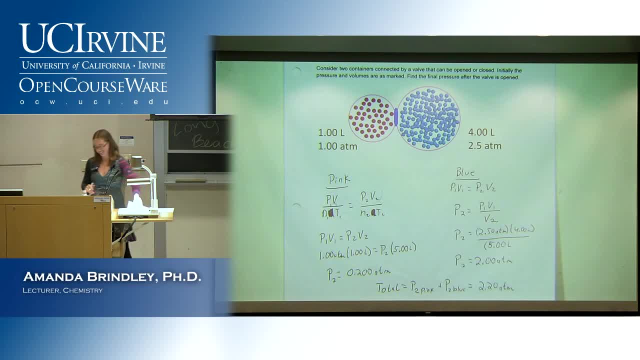 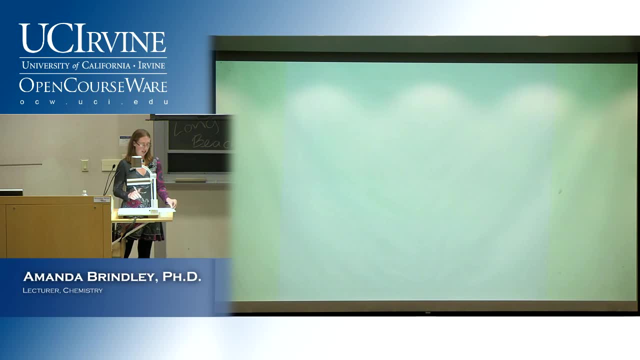 That was the real reason for doing it here. OK, I went from a little bit of a breather was the real reason for doing it here. OK, But I think you'll all be really happy that I'm doing this hard one and as soon as I put it up and you see the format, you'll see why. 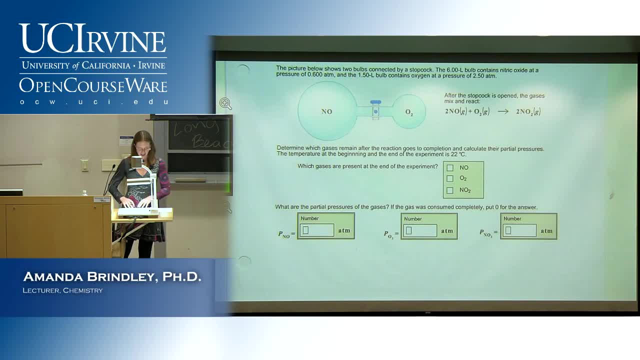 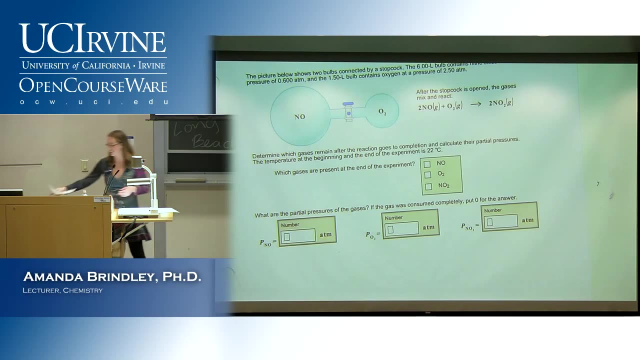 Any guess where I got it from? Yeah, not Wiley Sapling. OK, For those of you who don't know, Wiley is the other homework program that some of the classes use. That's where that came from. OK, Yeah, This is from your homework. So you have the worksheet in front of you. 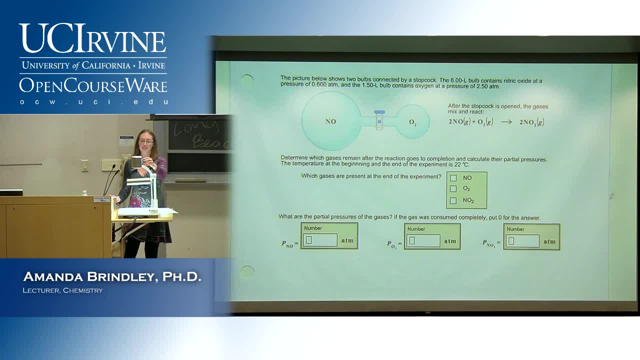 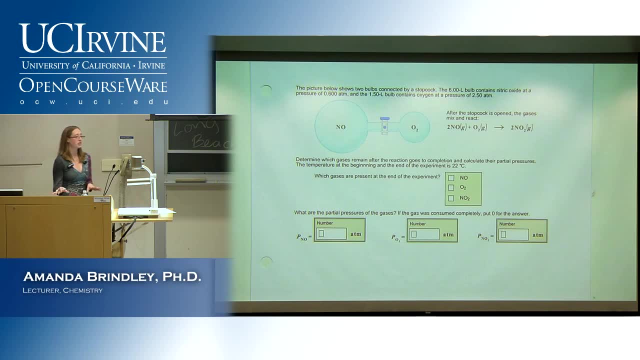 hopefully, because this is going to. you know, it's a long question with a lot of room, so I'm going to have to kind of zoom out and move around a little bit. But this is the same setup and that's why we kind of started with the easier version of this, and this is: 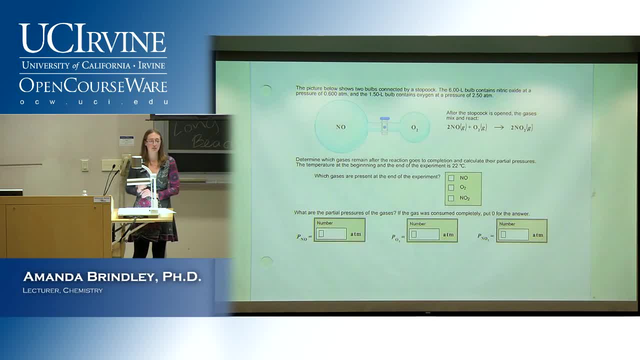 the more intense version of it. So we have NO and 02.. This is also my public service announcement. Remember all that fundamental stuff that you may have liked like said: well, I'm going to just remember this stuff. yeah, make sure you remember this. 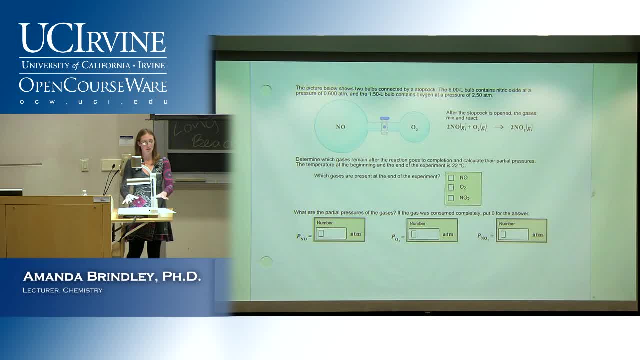 make sure you go back and do this, because this is a lot of the fundamental section that we sort of talked about a lot in lecture because- and I kept warning you- it was going to come back in chapter four. well, it's here. so we have two valves or two bulbs. they're connected. 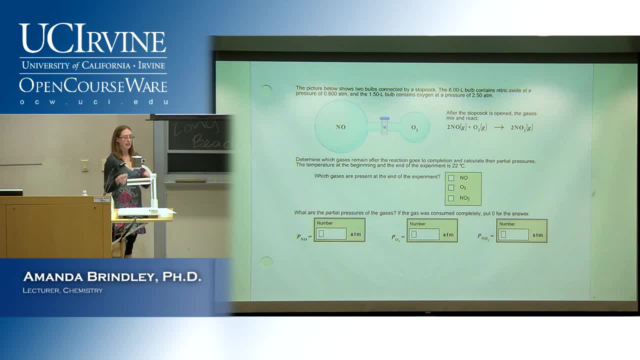 with NO and O2. in the last situation they didn't react. right, we just put them together, let them mix around and found a new pressure. but in this case they're reacting. they're forming a new substance, ok, and so it gets a lot more complicated now. now we have to. 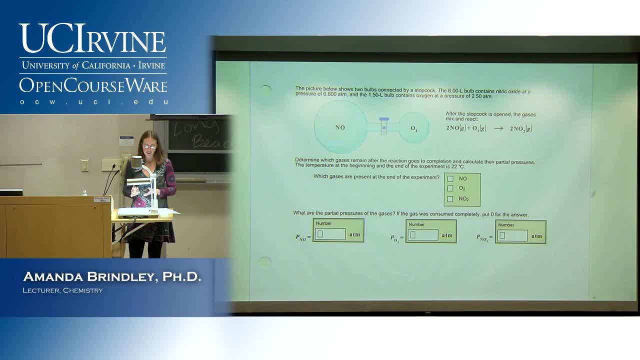 deal with a bunch of stoichiometry as well. so we need to find the pressures of each one. but to do that we have to find the moles of each one first. and to find the moles of each one, what do we have to do? are they going to react and completely form two NO2 and we're. 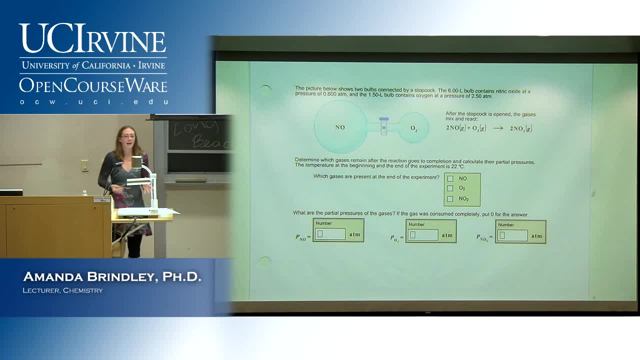 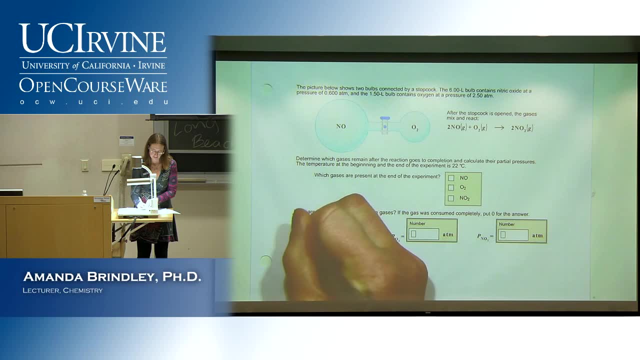 going to have none of this and none of this. no, what's probably going to happen? odds say that there's going to be a limiting reaction, limiting reaction. so that's our first step. ok, so we're going to find the limiting reagent. so we need to find the moles of each one of. 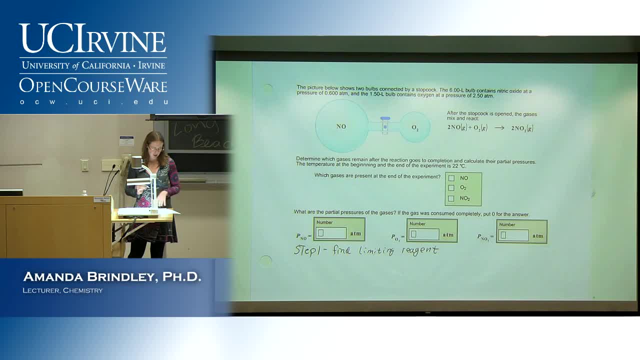 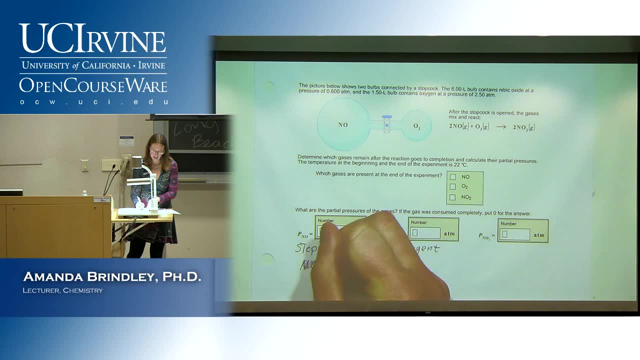 the starting. we need to find moles of NO and moles of O2. so that's our first step. so to find our moles of O2. actually, let's do moles of NO first. what equation are we going to use to find moles? 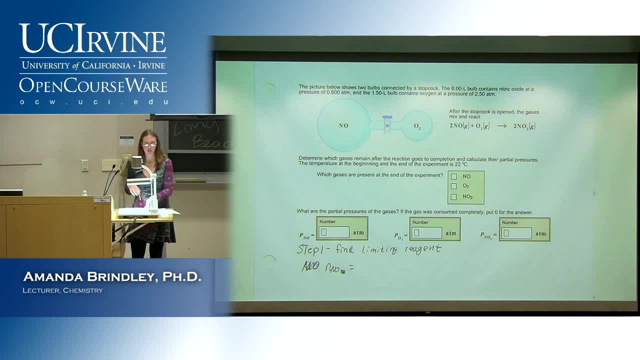 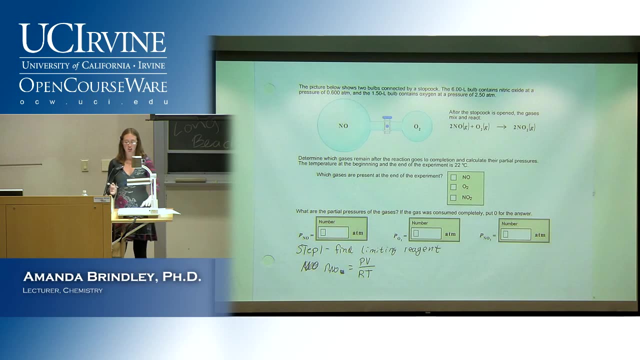 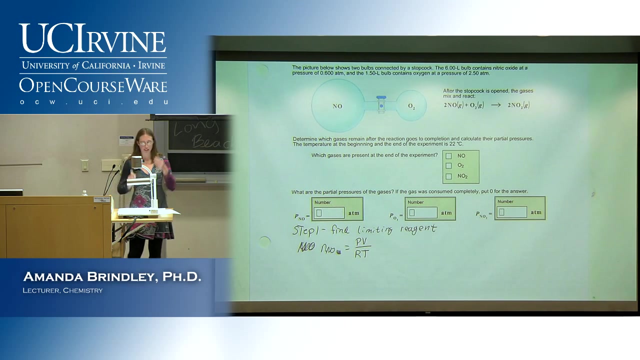 what do we have? we have some volumes and we have some pressures and we have some temperatures. so what does that sound like? ideal gas law? do we have to worry about our units in this situation? do we have R there? does R have particular units? yeah, so it's got to be atmospheres liters, right? so we're set there, so not a big deal. 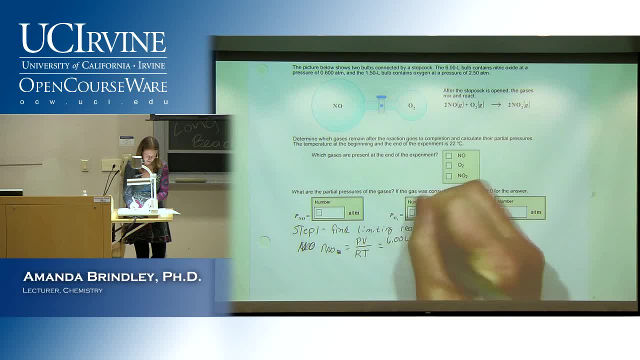 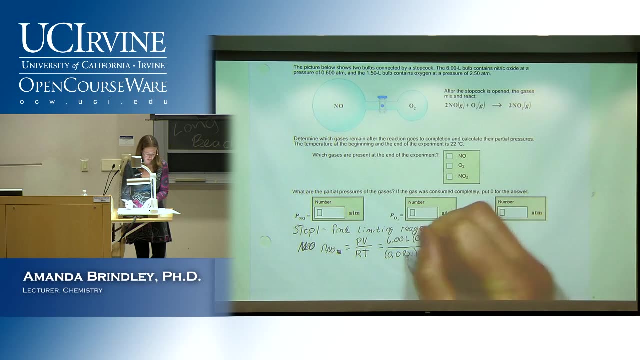 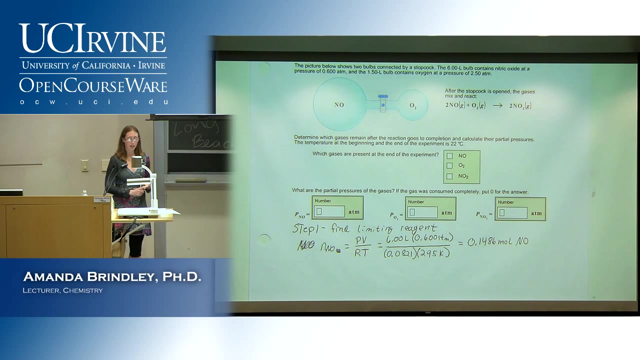 so we fill everything in. so this is all taken directly from the question. I'm skipping the units on R because, honestly, we're really short on room here. ok, so we're going to have that. that's just calculator button pushing and we get this. ok, so that's our moles of NO. now what do we have to solve for? 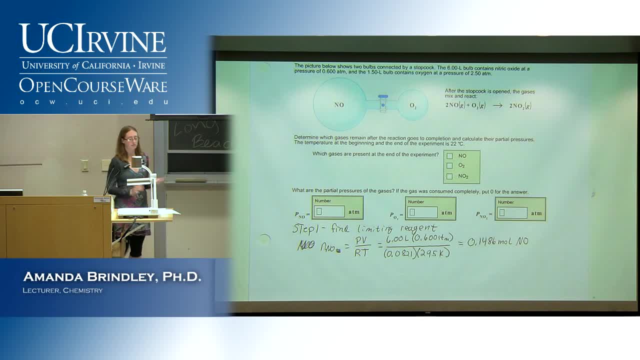 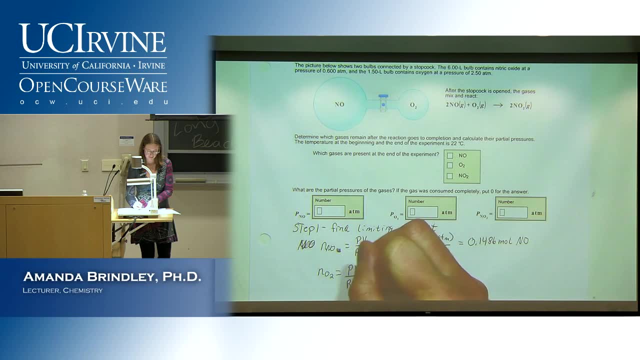 well, if we're finding a limiting reagent, we need moles of the other one, right. so exact same thing. And Sapling was nice and only gave you everything in the right units. on this very, very long, hard problem, I decided I didn't want to be nice to you on the previous one where I did that, so OK. 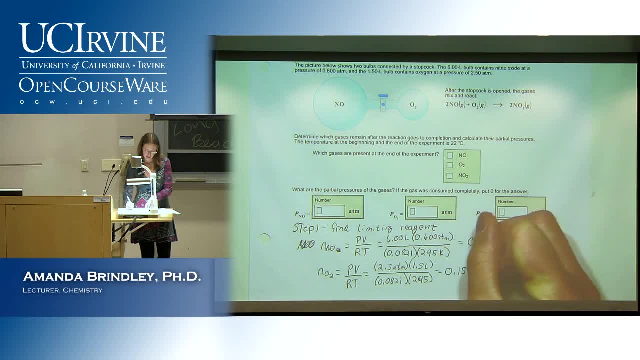 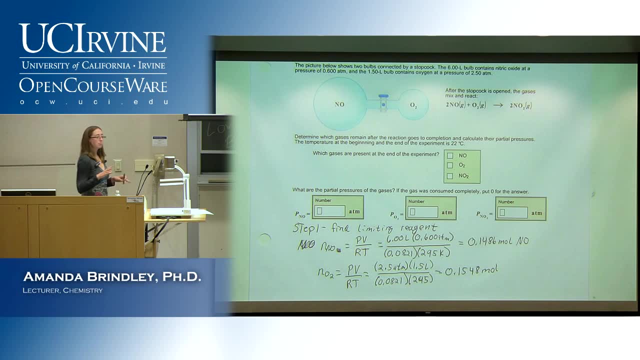 So we plug this in, OK. So now we come to limiting reactant stage. There's a bunch of different ways to do limiting reactant and everyone has their favorite way. I think in this one, doing logic is the best way. You can choose to do it mathematically if you want. 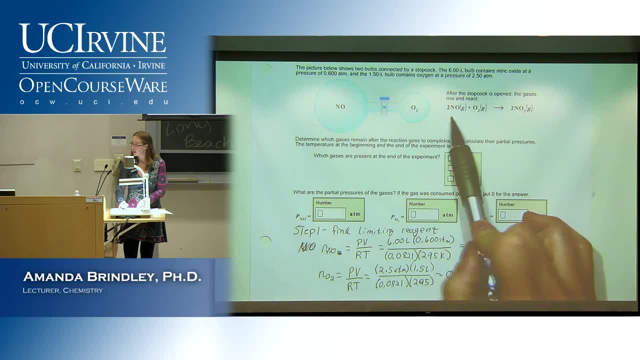 The two kind of are hand in hand. So if we look at this, if we have one oxygen, how many NOs do we need Two? If we have five oxygens, how many NOs- Ten, Ten- If we have 20?? 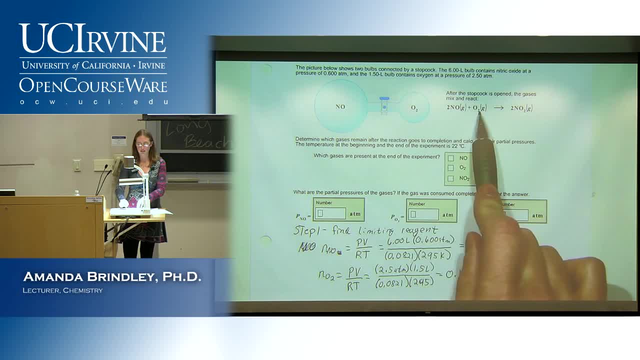 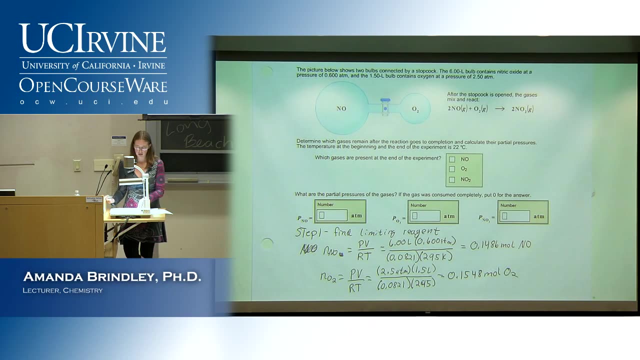 Forty, Forty. So we've got the pattern right. How many do we need Double Double Now, do we have that? So we look at oxygen. Do we have double the amount of NO that we need No? So what one's going to be our limiting reagent? 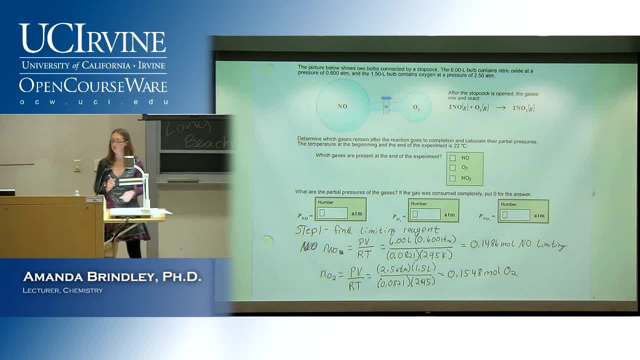 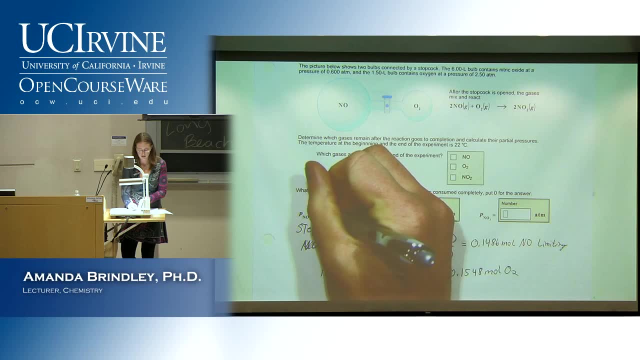 OK, All right. So how much NO are we going to have at the end of this reaction? Zero right, So no moles, no pressure. OK, Next part, then We need to figure out how much NO2 we're going to have and how much what else are we going? 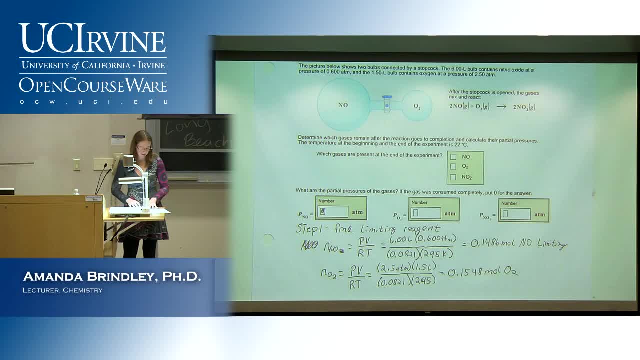 to have. Are we going to have any oxygen left? Let me reword the question So: which one was our limiting reagent? again: NO, So that means that we have more oxygen than what we need, right? Yes, OK, OK. 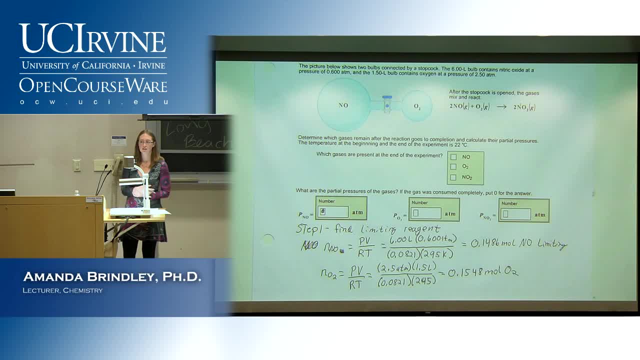 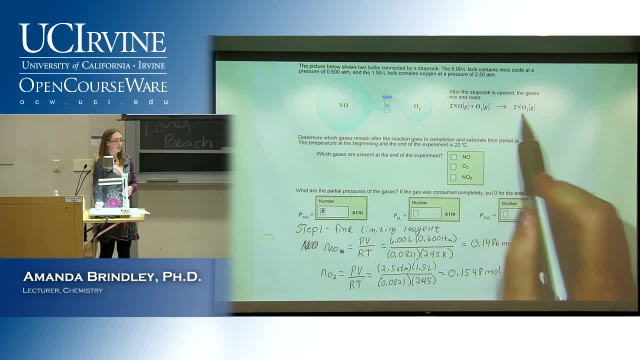 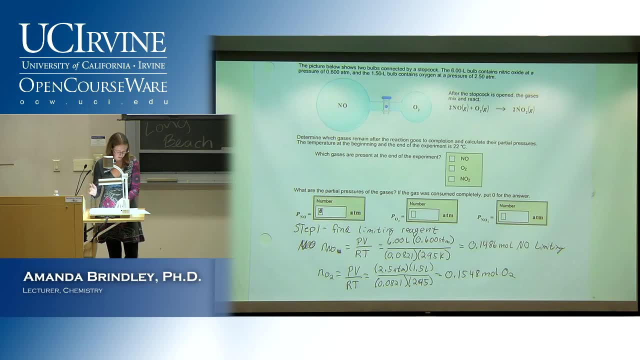 Yes. So we're going to have to figure out how much NO2 we make and how much oxygen we have left. So that's our next goals. So it doesn't really matter which order you do it in. I think I found moles of O2 first. 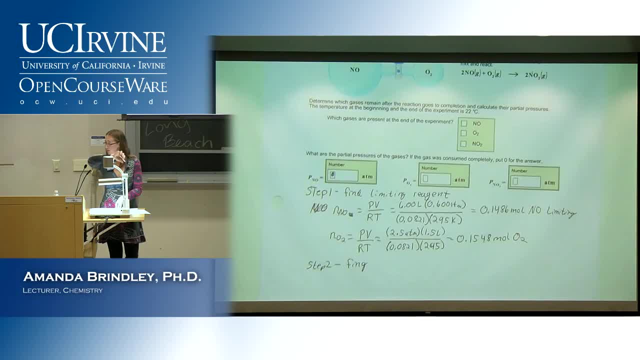 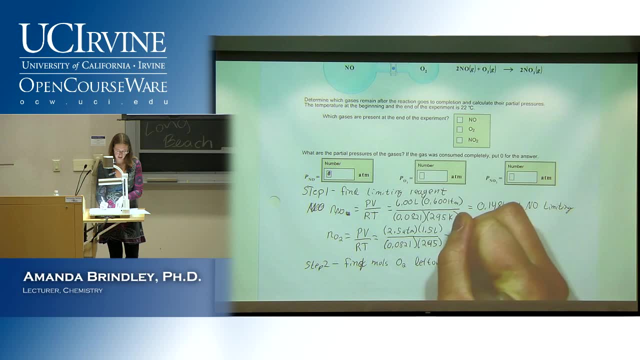 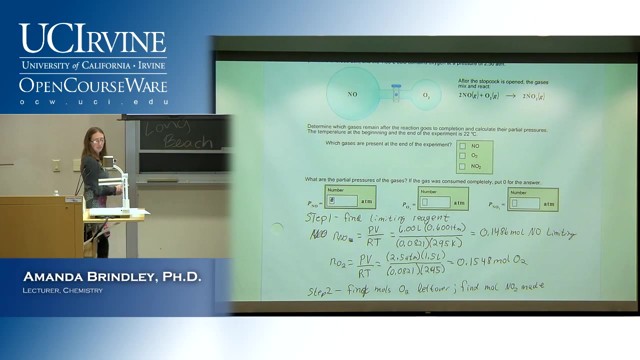 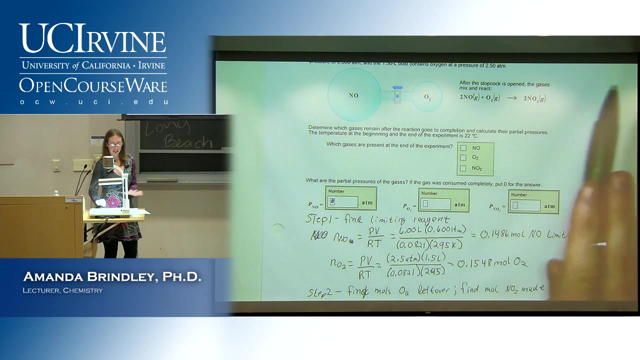 So we're going to find moles O2 left- OK- and find moles of NO2 made- okay. let's do NO2 first, mostly because it's the easiest. so if we used up all of our moles of NO, how much NO2 did we make? let's let's break it down. 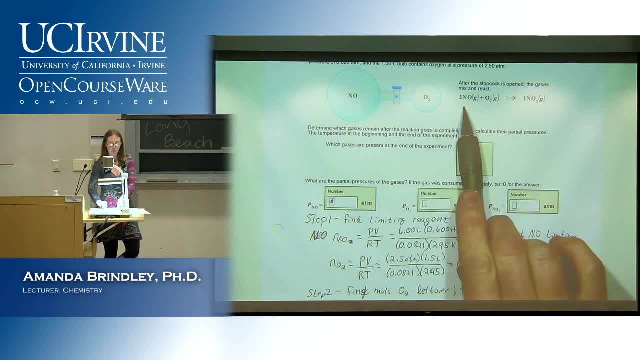 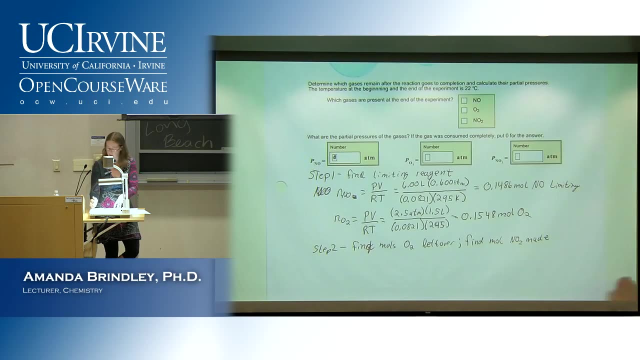 a little bit more. let's say I make one mole or I make one. I have one mole of NO. how many moles of NO2 would I make one? if I had five, I would make five. right, they're the same, and that's because the coefficients are the same. so what we're going to do here is: 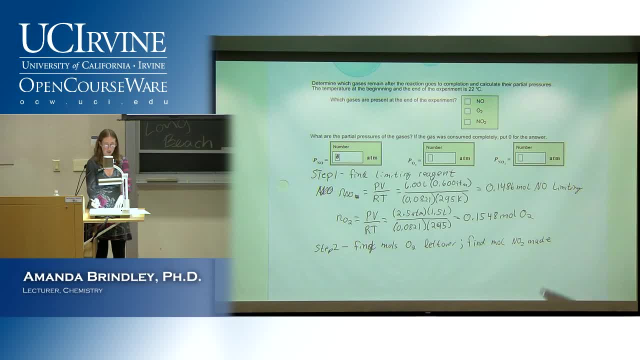 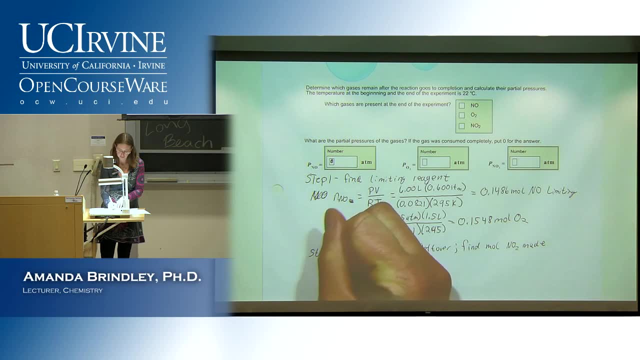 if we know how much NO2 is made, or we know how much NO we started with, which we do, we know how much NO2 is made, it's the same amount, okay, okay, so we just write it down. basically, we just take our amount of NO we started with and 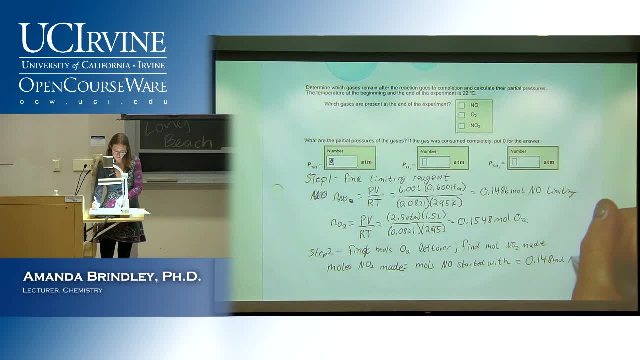 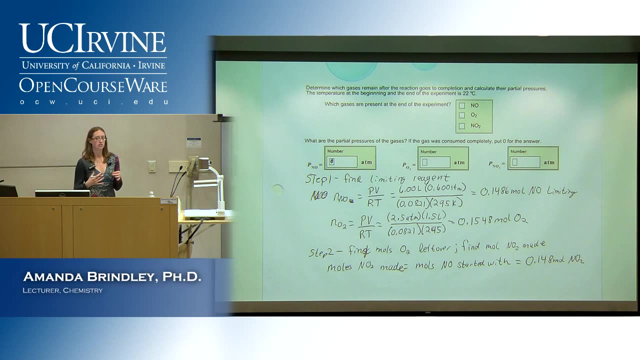 we write it down. okay, now, oxygen is a little bit more complicated. right placed, anything higher than Catholic, although not yeah, because we know how much we had to begin with. and what can we calculate that happened in this reaction? How much we made, how much we used up, how much is left over? what can we do with one? 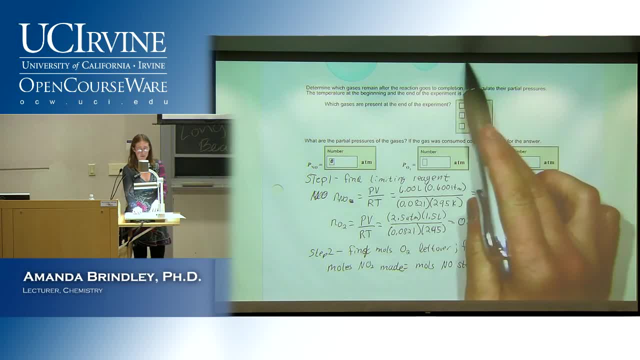 calculation using this reaction. How much was used up? right We can we know that, for if this has two, that one of them is gonna get used up. if we have five or ten, that five of them are going to be used up. okay? 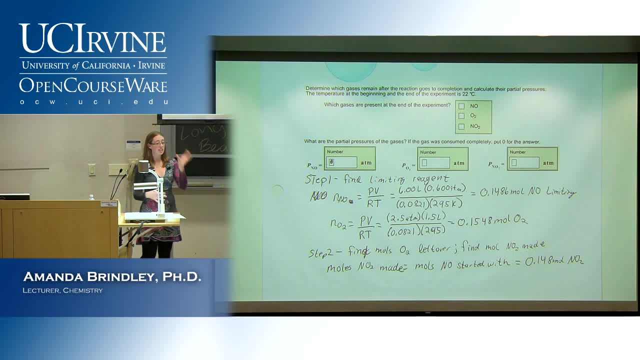 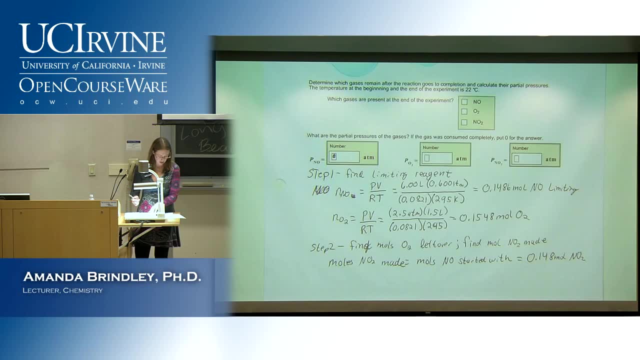 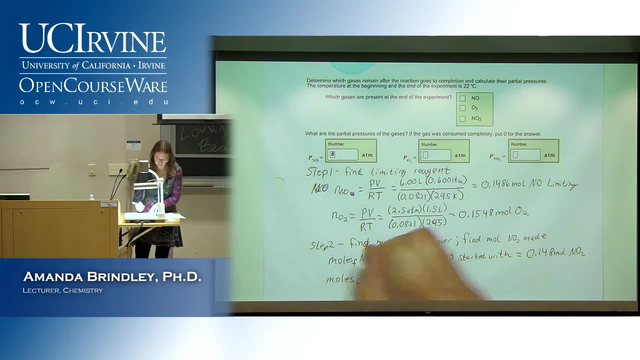 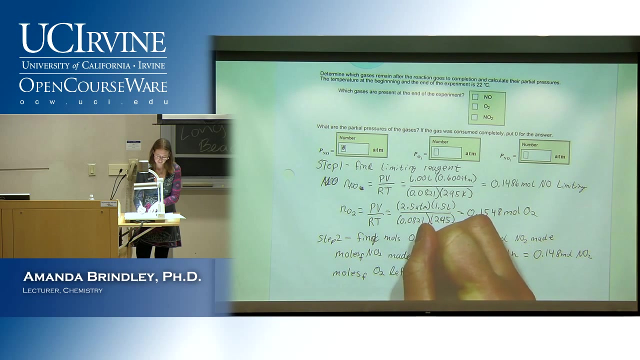 Oh, okay, to find our final amount of oxygen, we're going to take our initial amount and we're going to subtract away the thing that we used up. So let's do that And let's just put a little F underneath moles for final, Just to make it super clear. So, obviously, if like 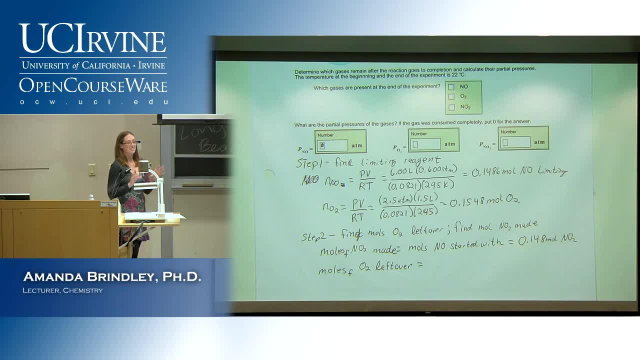 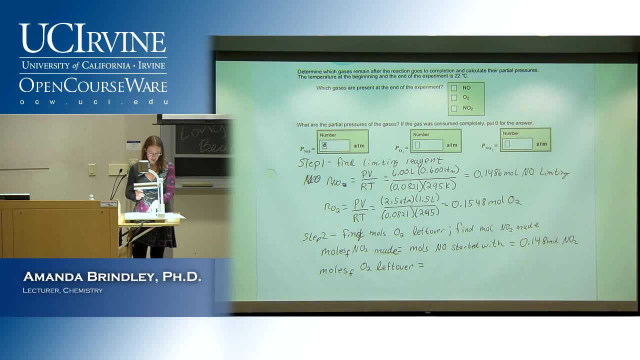 I were to give this on an exam, you wouldn't need to write down all of these sentences. I'm just doing that for you. so when you go back and look at this, you know what's going on. So moles of O2 left over. How much did we start with? We started with this right. 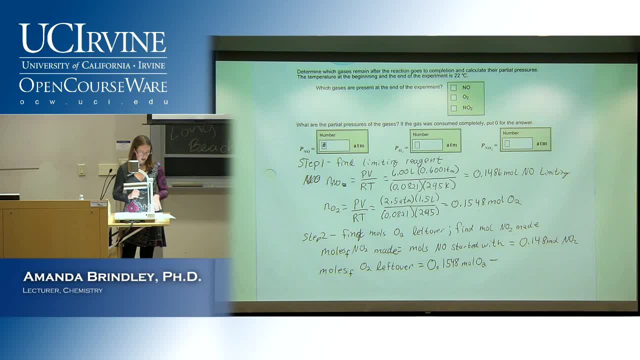 And we're going to subtract what was used. OK, How do we figure out what was used? Well, we know I'm going to kind of do this. OK, How do we figure out what was used? Well, we know I'm going to kind of do this This. 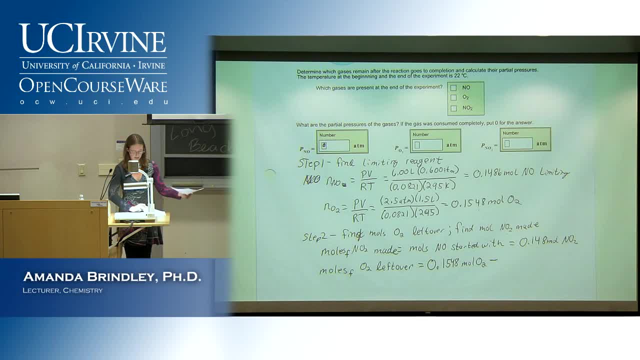 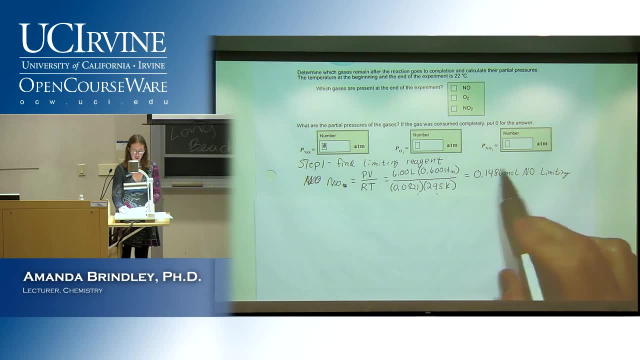 is as a sidebar, like I do sometimes. We know how much NO we started with right Now. how is the moles of NO and the moles of oxygen related By the mole ratio? So writing this out really big so that you can see. 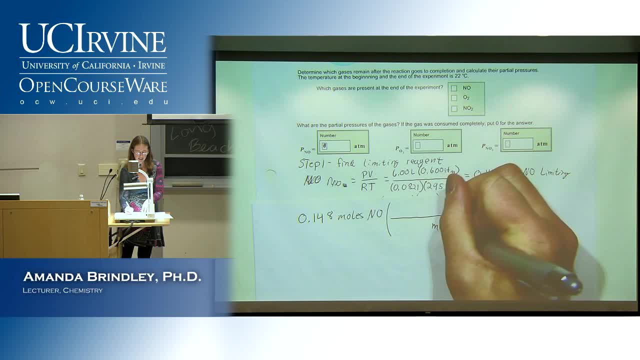 And then I'll plug it into the smaller area. Just want to make sure everyone can see. Our moles of NO will go here, Our moles of oxygen will go here. And what is the number that goes in front of the oxygen? One, We got that from where The equation Here is two. OK, 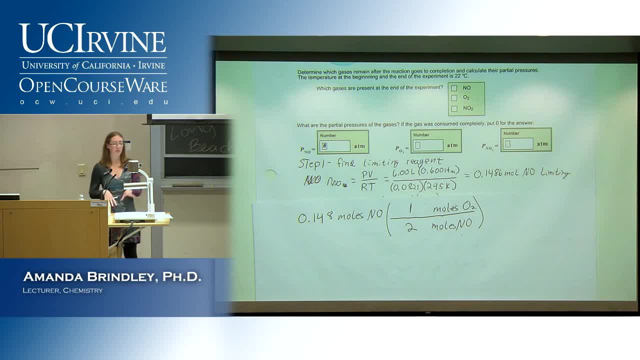 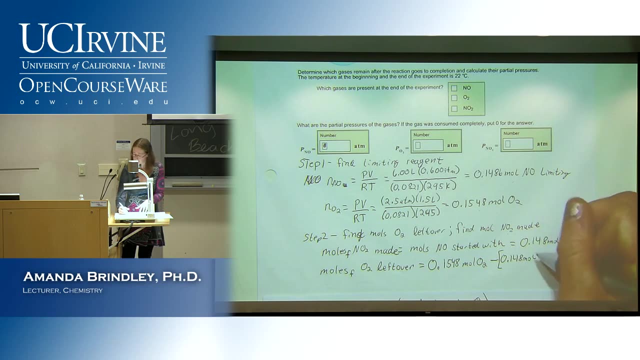 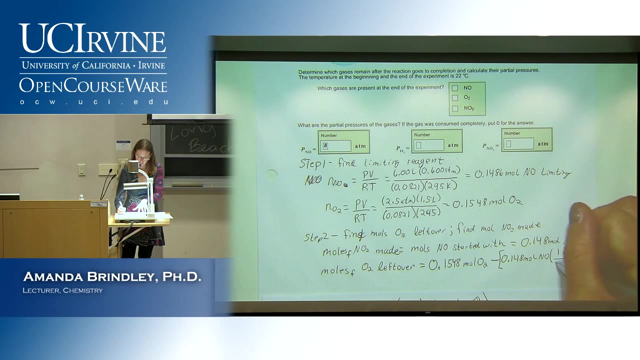 So I just wanted to write it out big and then I'm going to fill it into the equation on the notes we've been taking as well, But just because it's getting tough to see. OK, So we took our total, that we started with our initial amount And we subtracted that. 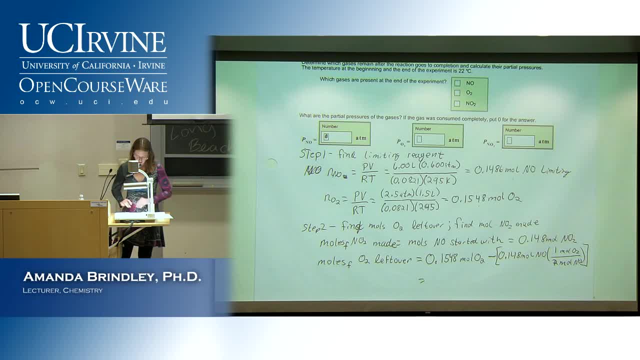 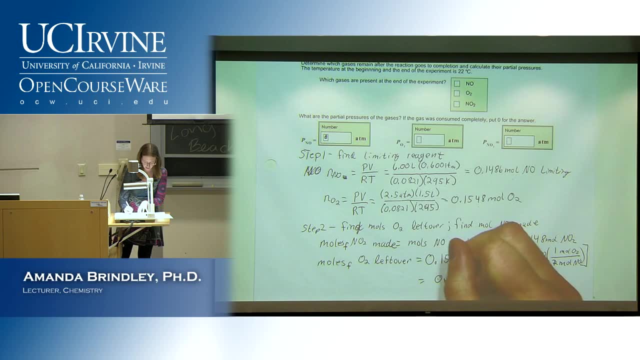 subtracted what we used, And when we get this, then we end up with 0.081.. Ok, so now we have our final moles of oxygen, we have our final moles of NO2, and do we have our final moles? 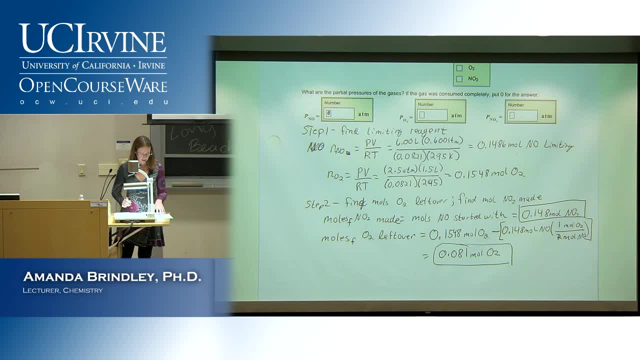 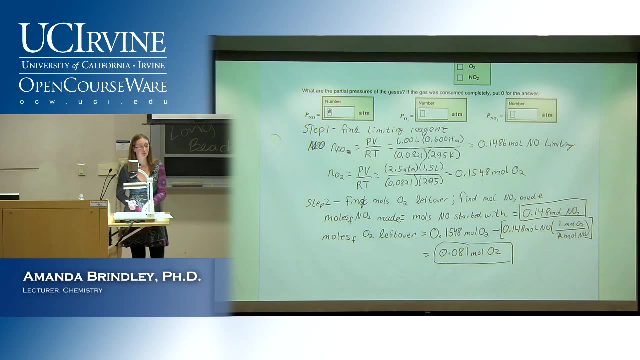 of NO, It's 0.. And so we're good there. Now, what equations do we use to go ahead and solve? Now we're back to the exact problem that we had before, The problem where the question of that's it got asked. right Now we're at the P1V1 equals or P1V1 over N1T1 question. 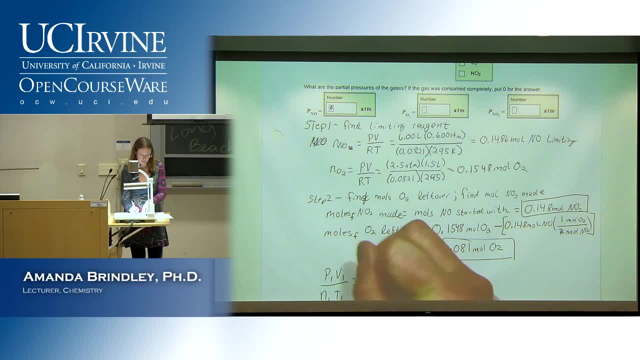 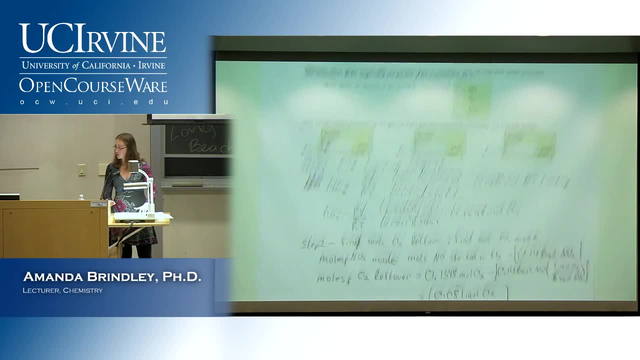 Ok, so now we're at the P1V1 over N1T1 question And we have to look at what's changing. So if you, you know, go back to the question and we can look at everything that is and isn't changing, we can fill everything in. 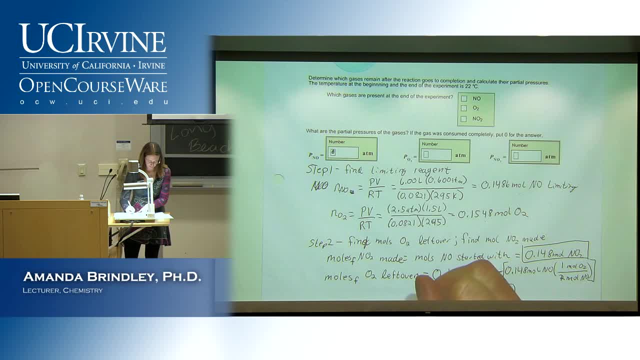 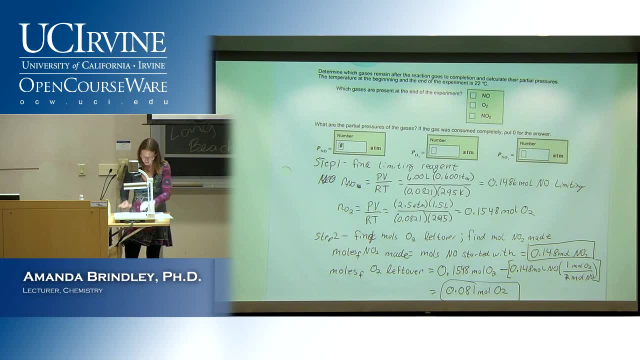 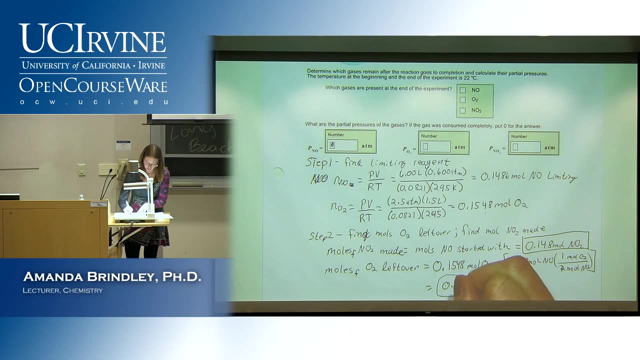 Ok, so let's see we're still doing ok for time. Ok, so when we go to do this, we put in our final amount of moles. oh, ok, so now we're at the P1V1 over N1T1 question And 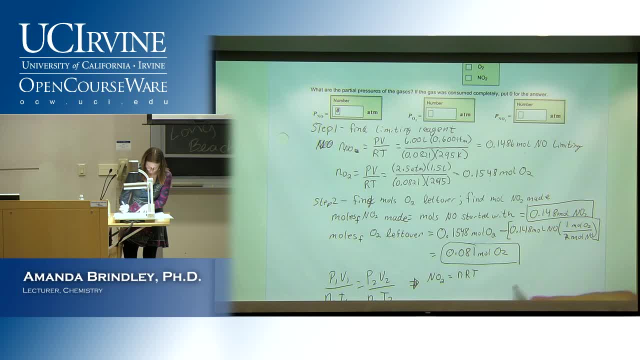 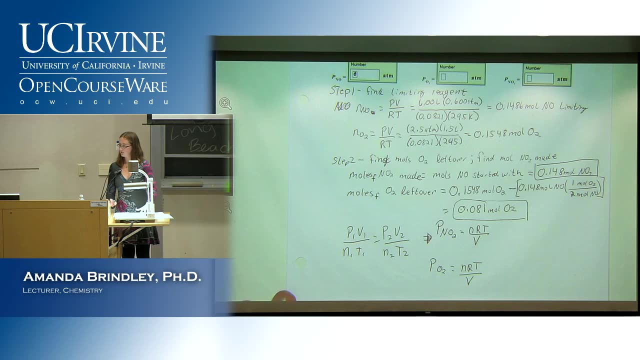 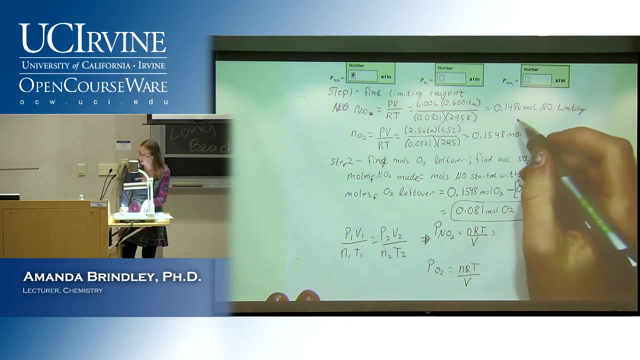 we'll fill everything in. Thank you, Okay. so we do this for each one. Is that too…oh, that's okay, You guys are alright And we fill everything in. So now this becomes a scavenger hunt. right Now you have to go. 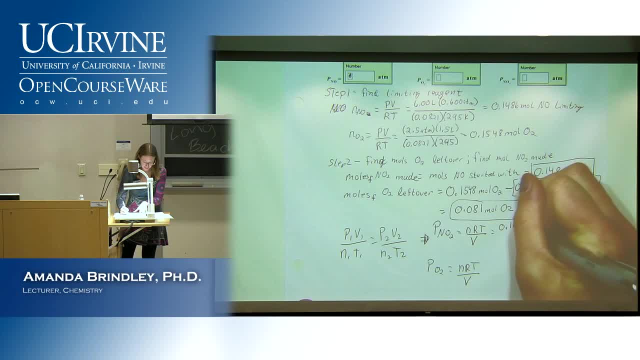 through and figure out where everything is coming from. Thank you from. Make sure you grab all your final values and not your in between values. So this is just R. Make sure you remember, after all of this work that you've done to convert your. 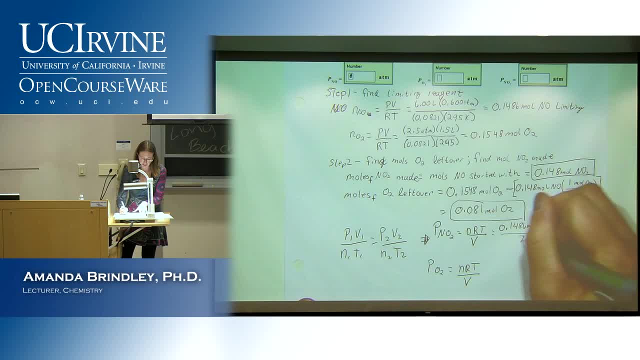 temperature to Kelvin. right, Because it's easy to forget things like this after we've gone through everything. We're going to walk through it a little bit here once I finish it as well, and so we can talk back over everything that we did. So now I'm just filling in numbers. 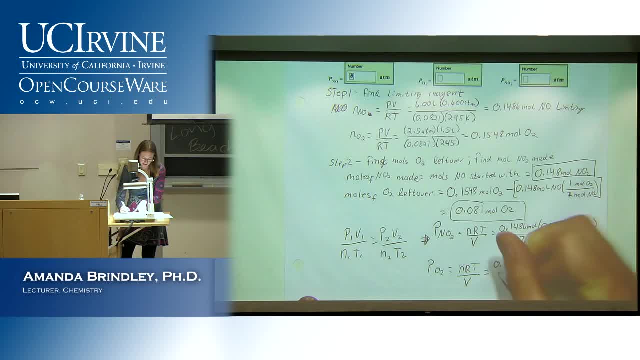 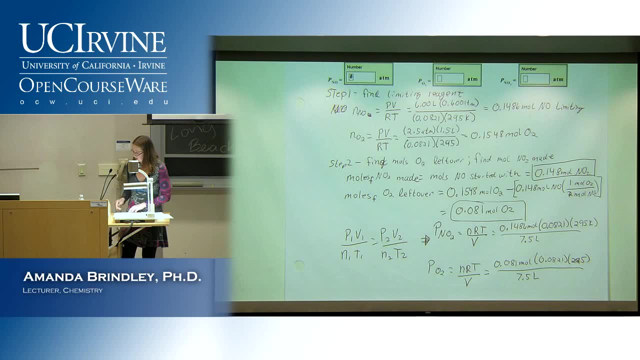 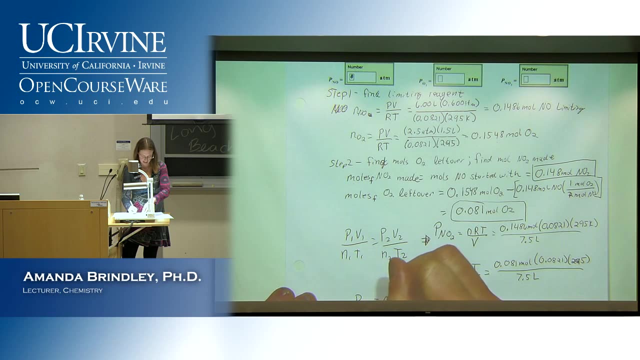 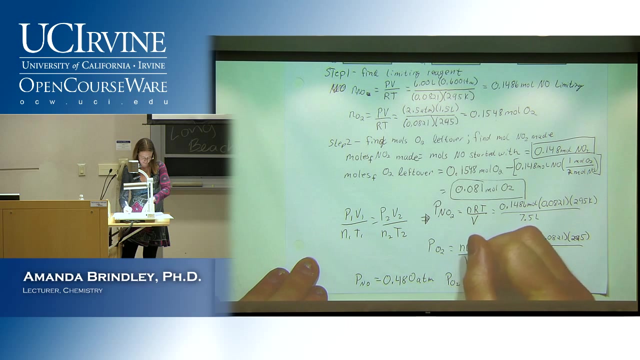 We've done all the hard parts and we're filling everything in. So when you fill those into the calculator, I ran out of room so I can't write it beside it Now. of course you know that your homework values are going to be different than this. 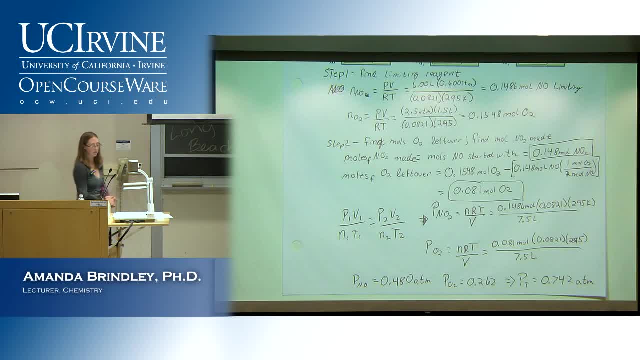 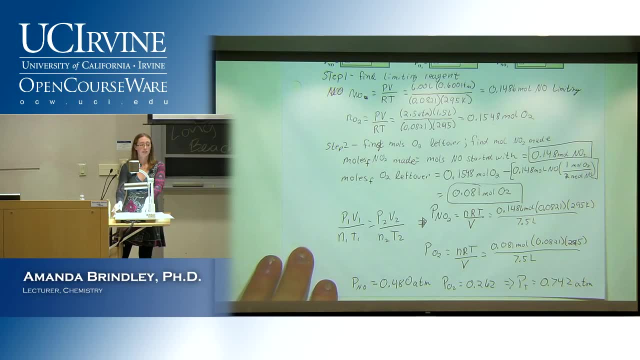 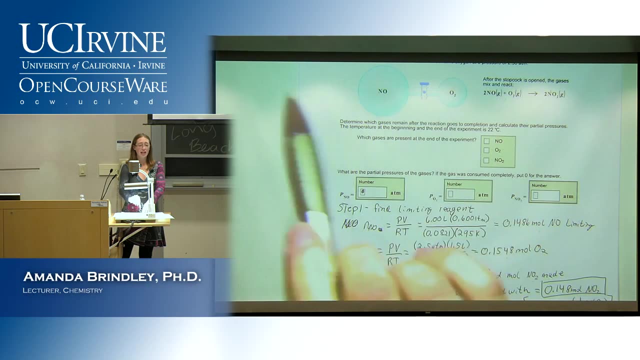 so don't go filling those in right away. right, You know, something changes your numbers on you, So that's your total pressure. Let's go back through and talk over what we just did in the last like minute and a half. OK, So we started by saying: well, in order for me to find the final pressure I need, 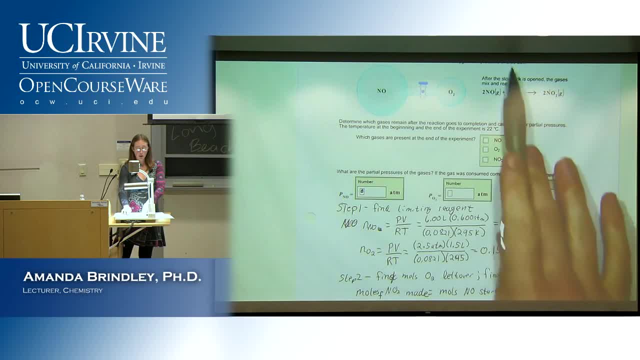 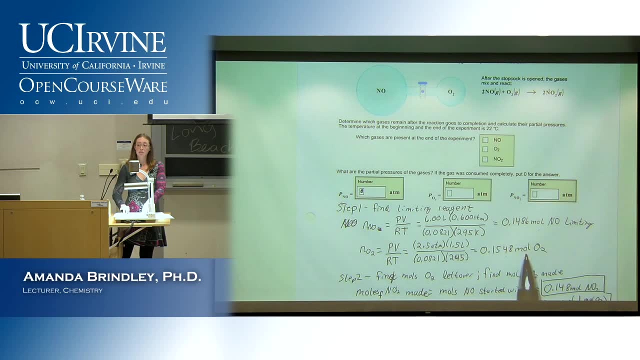 to find the initial pressures. So I know all of this detail. I can use: PV equals nRT and I can solve for my moles. Once I find my moles, I can use all of my knowledge that I remember from the first week of class and I can use stoichiometry to solve for one. 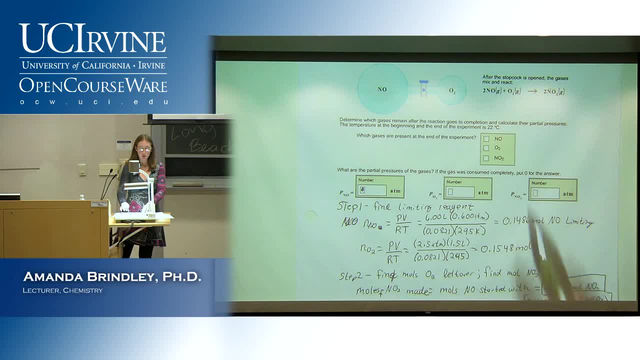 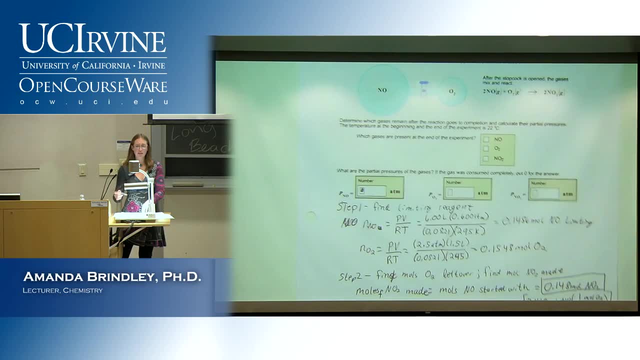 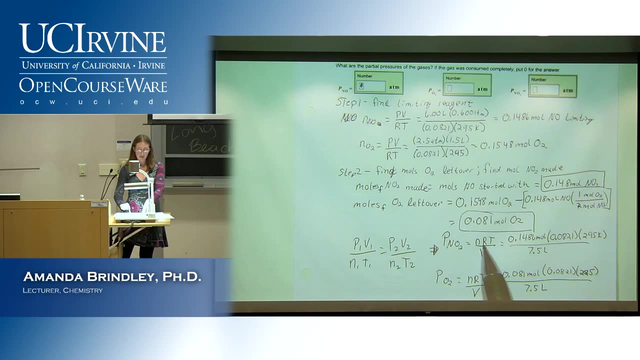 the limiting reagent. so I know what's not going to be there. Two, how much of the non-limiting reagent is left over, and then how much of the product I made, And then, after we have that, we have our moles of everything. So we still know that we have R equals nRT plus. 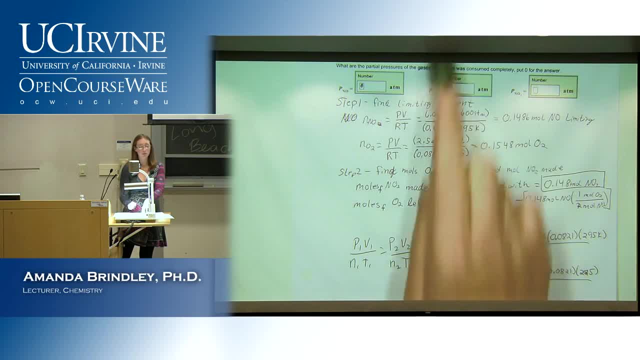 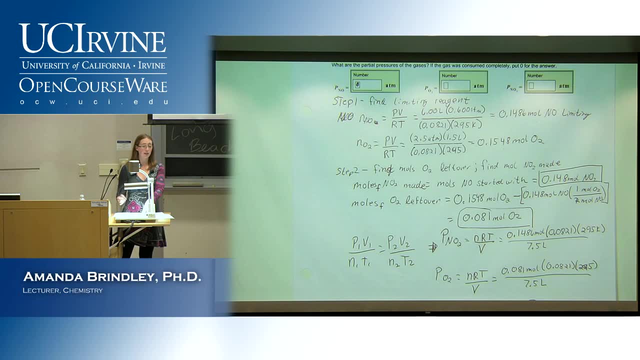 R and T and V. We can find that from the problem. But now we found our final moles and we can fill in our final moles into the PV equals- nRT equation again. So really, at its heart, what this is doing is it's taking and it's using, you know, conversion factors, just like 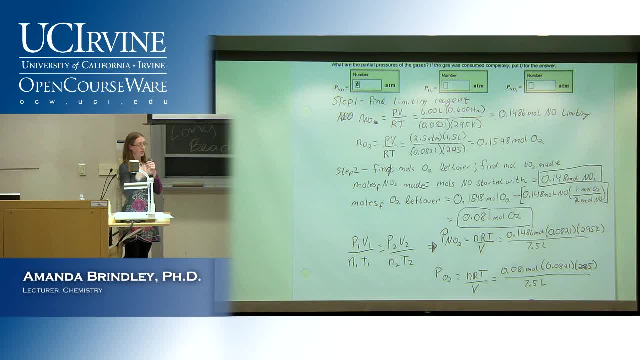 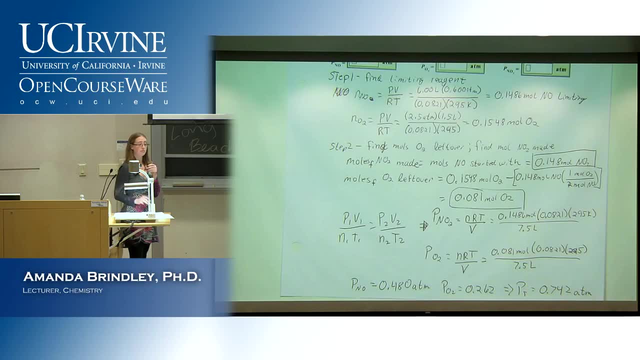 we did before and you have to go through moles. So you convert everything to moles, You do your stoichiometry and then you convert everything back into pressure And I'll leave this up as you guys are packing up and stuff, so that you can see it if need be.